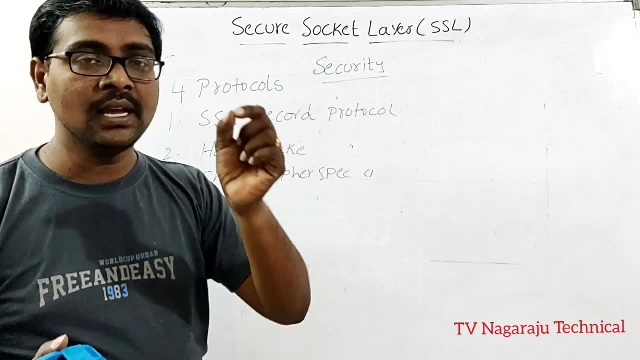 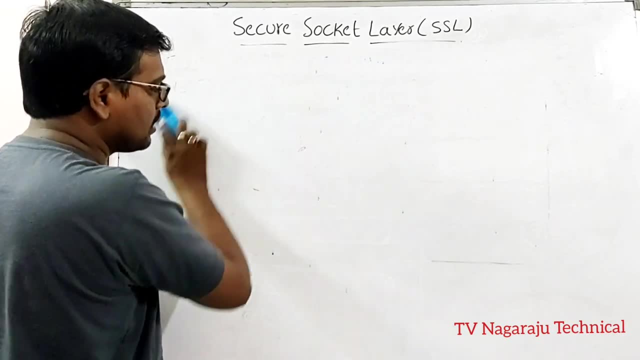 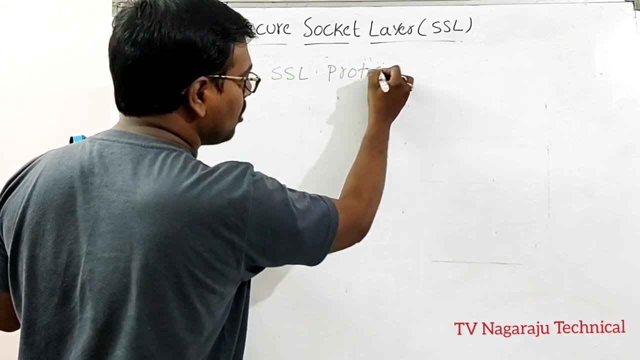 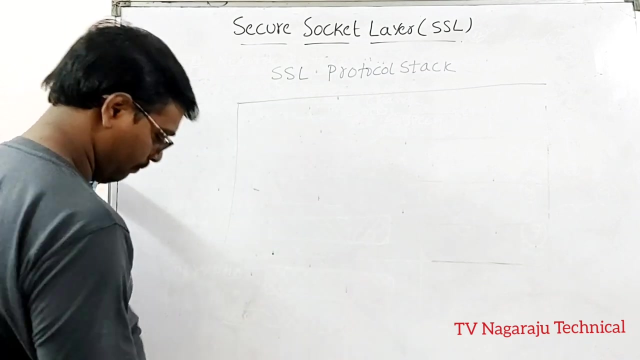 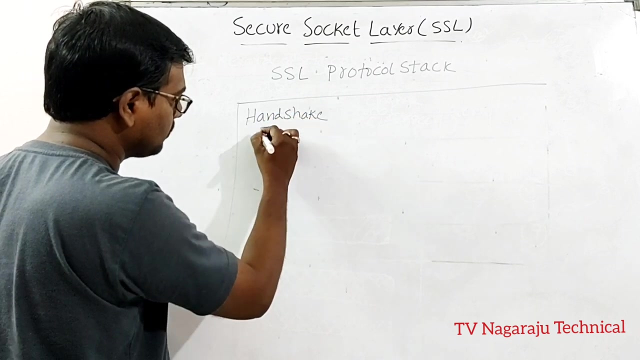 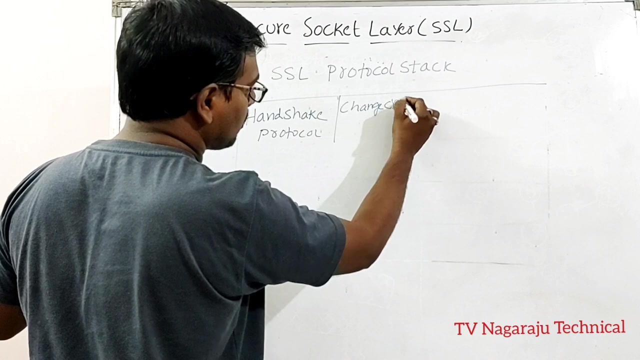 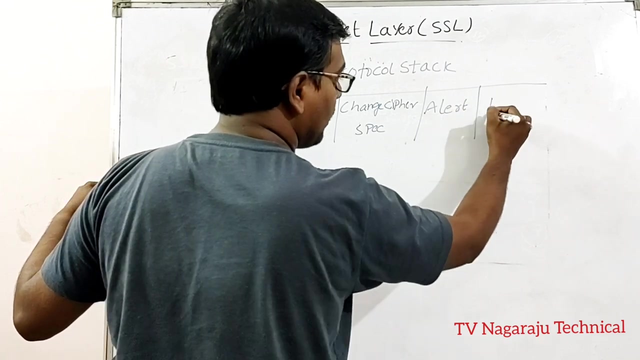 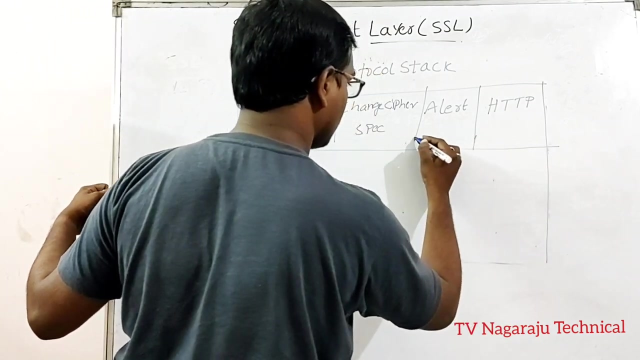 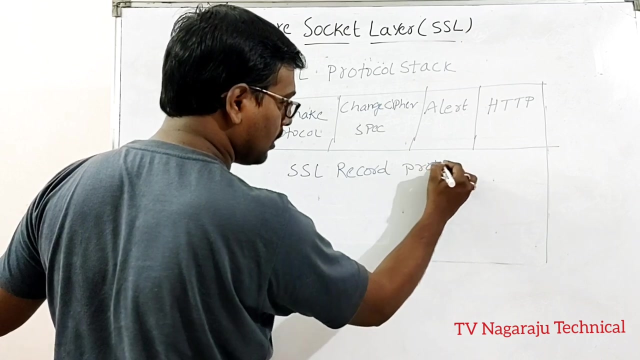 the protocols are stored by using SSL protocol stack. I will show you the diagrammatic representation, The same protocol. They are represented as the SSL protocol stat. so first one handshake protocol, change cipher spec protocol, change elect protocol and then HTTP and then HTTP here, SSL record protocol. SSL record protocol. 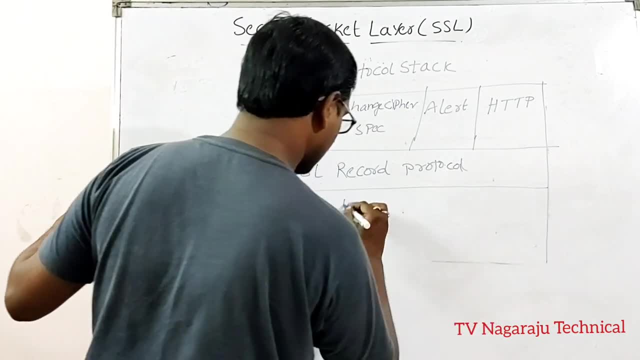 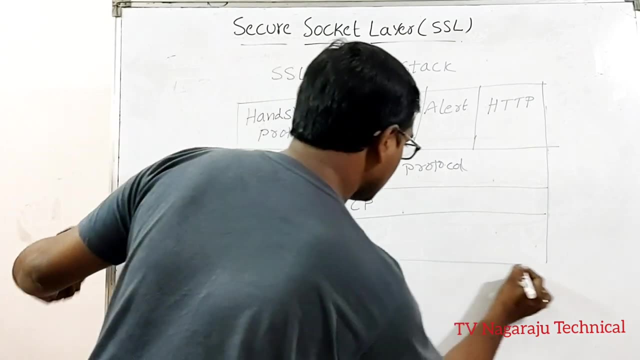 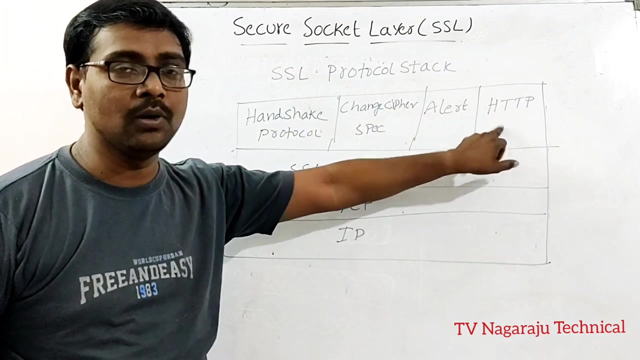 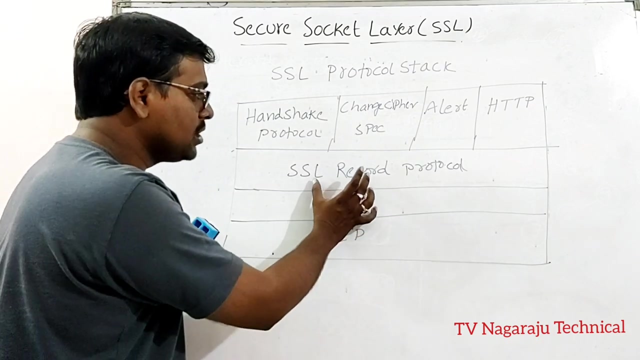 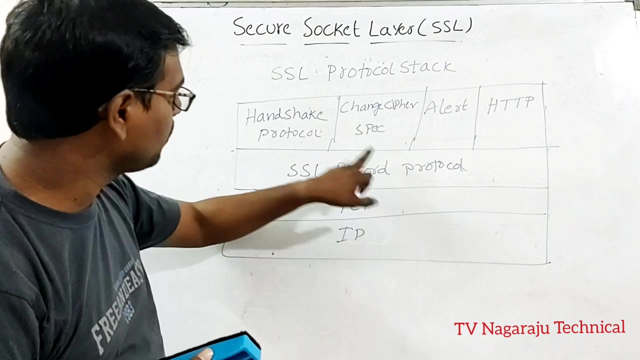 TCP IP. so generally, this SSL record protocol is above the top of the TCP and bottom of the below the HTTP. this is called SSL protocol strap. now I will explain each and every protocol in detail. so what are the four protocols? you need to write SSL, the record protocol, short��을, protocol Change cipher set. 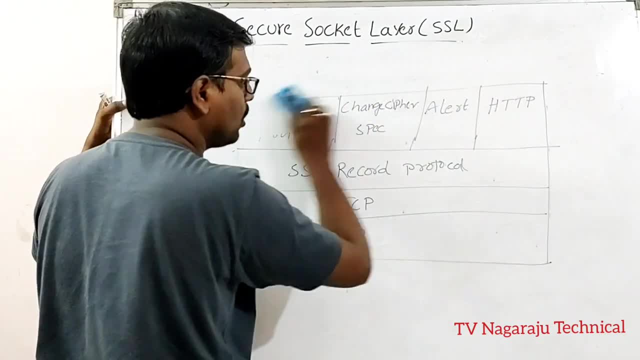 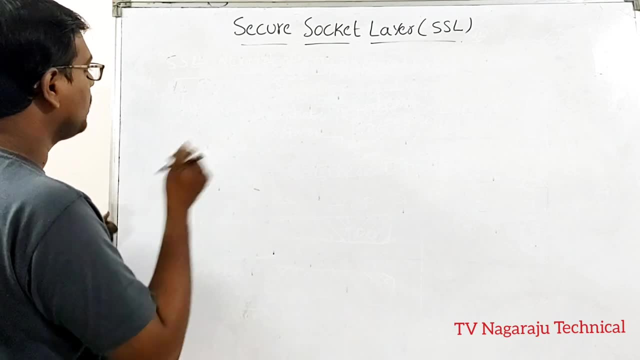 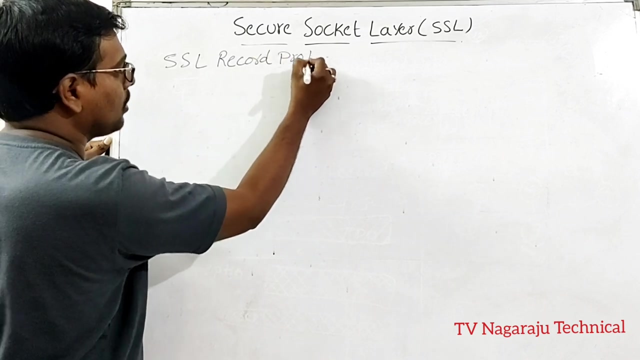 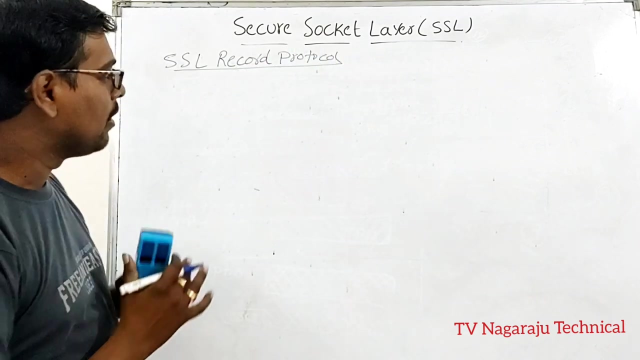 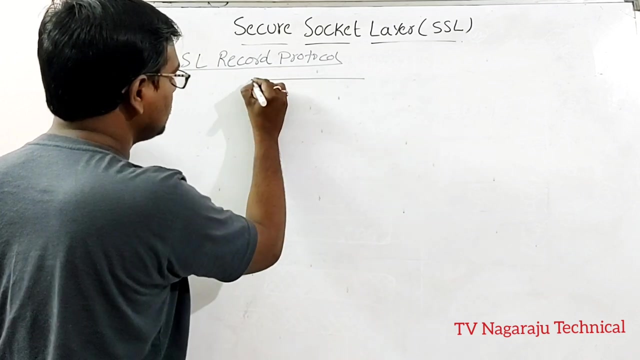 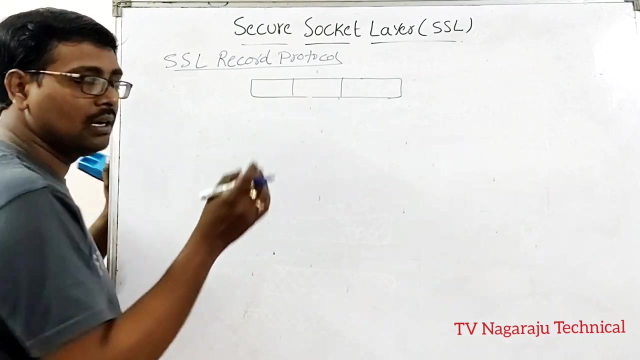 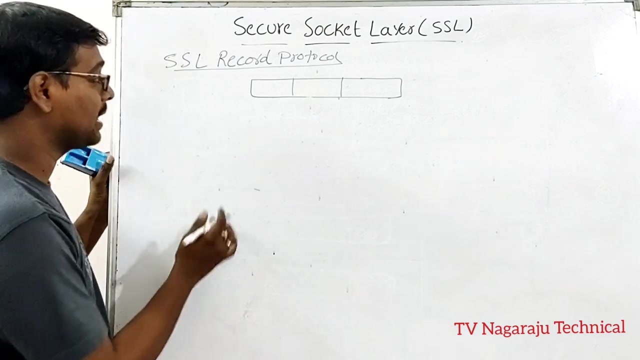 and Alert. so, coming to each and every protocol in detail, Very simple topic. the first one is ssl record protocol. so what happened inside this SSL? So an application data is given. So the first step is assume this is my application data. An application data is given. Generally, the application data is divided in terms of blocks, or also called as fragments. 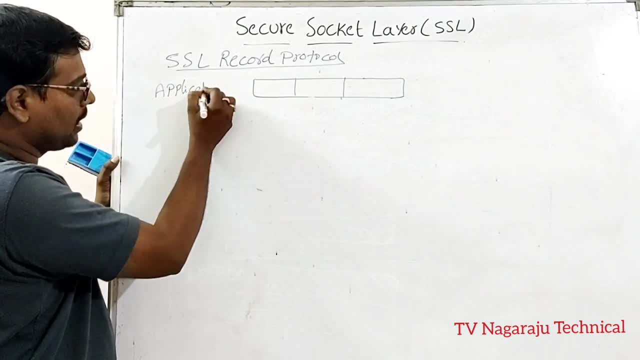 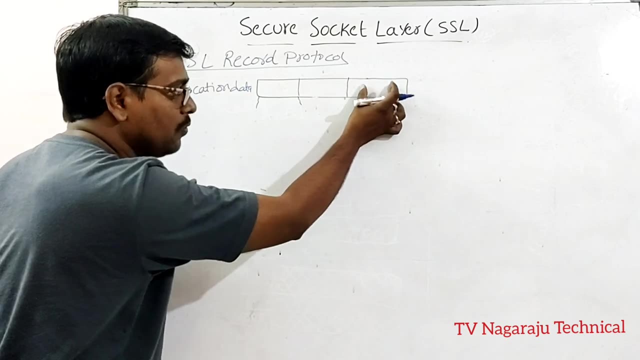 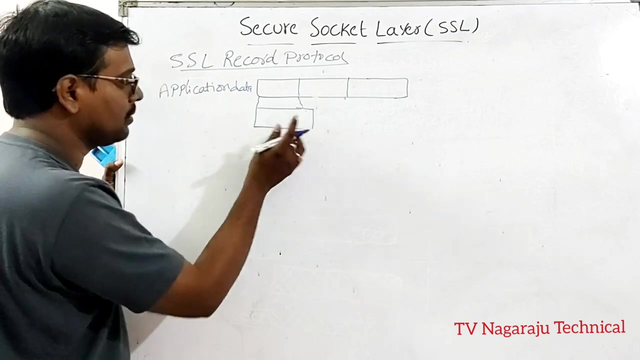 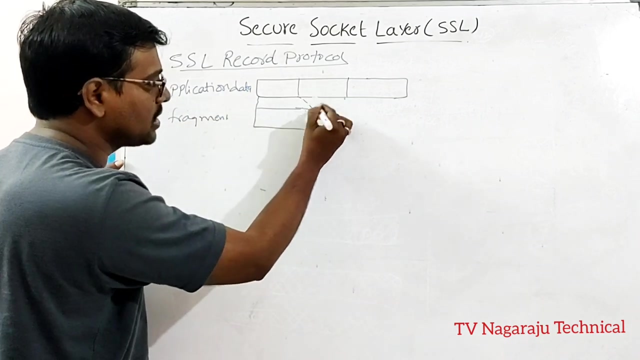 So this is my data. This is my data divided into fragment 1, fragment 2, fragment 3 and so on. For example, for understanding, consider one fragment. Assume this is one fragment. Each and every fragment. we are doing the same process. Each and every fragment, we are doing the same process. 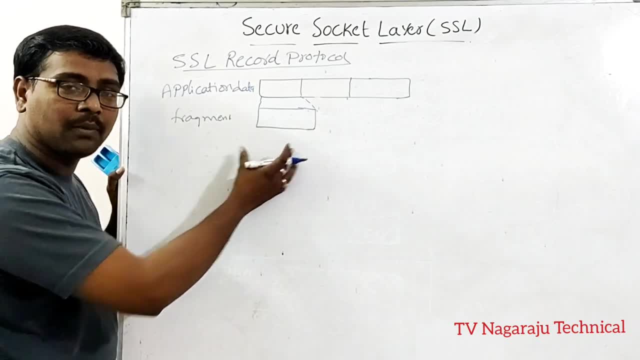 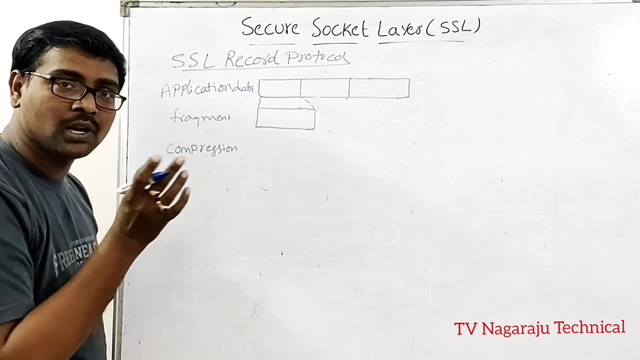 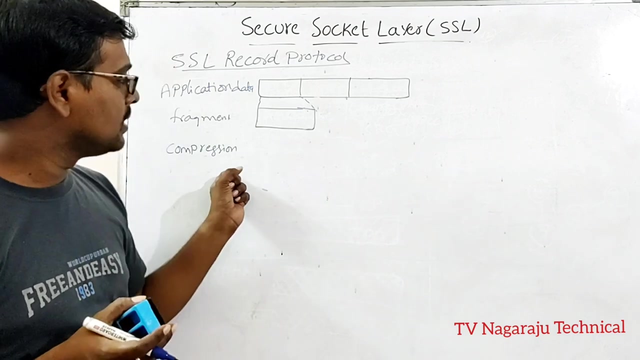 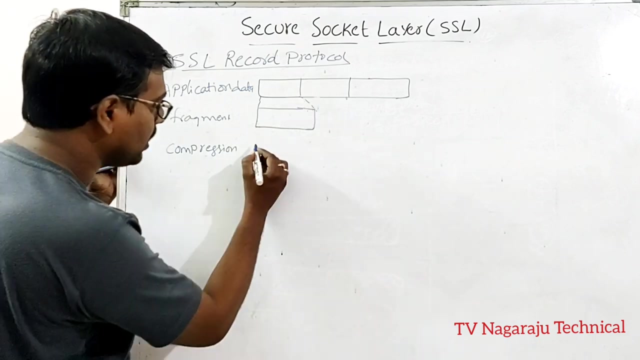 Okay, Once I received the fragment, what are the steps Here? first one is: you are applying some compression algorithm on the fragment. Anyway, this compression is optional. Anyway, this compression is optional. If you want, you can apply the compression on the fragment. Now, see this one Suppose: after applying the compression: 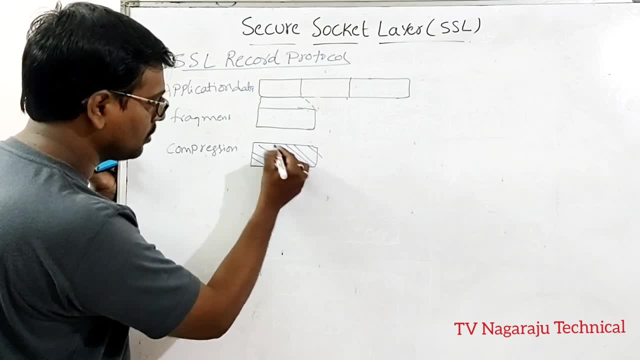 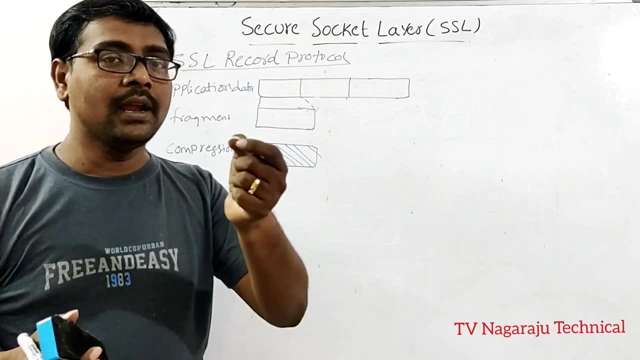 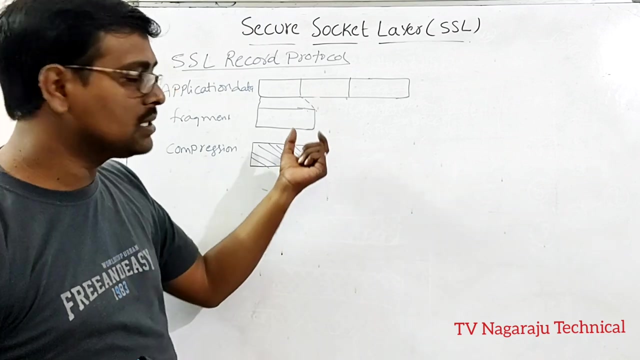 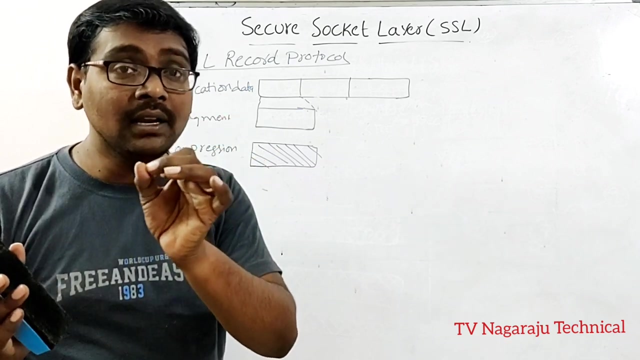 So the fragment is compressed. Now what is the next step? Apply any secure hash algorithm, SHA algorithms or MD5 algorithms on this compressed fragment, which is used to generate the message authentication code. Now, what is the next step? You need to calculate. 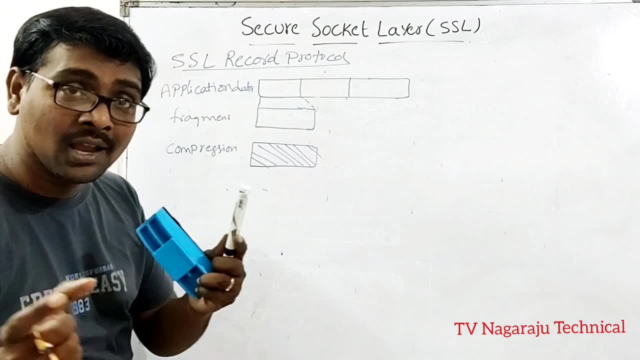 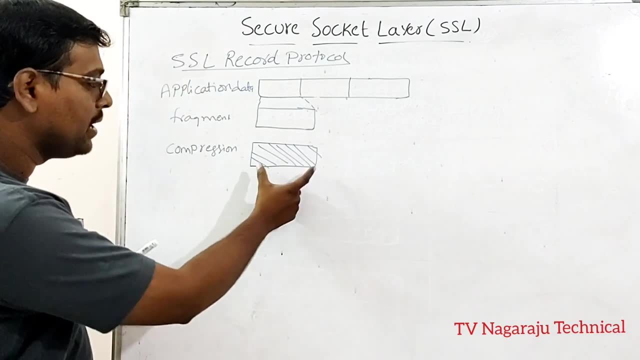 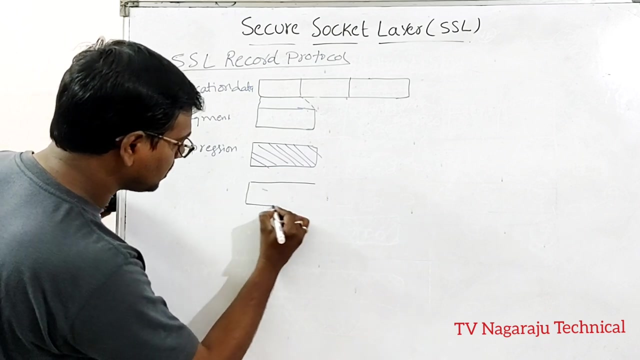 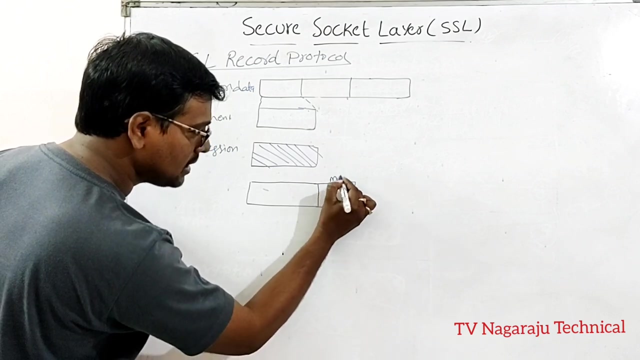 The message authentication code. Okay, Once the message authentication code is generated, We are getting the code is appended to this compressed fragment. Now see this one. What is the next step? This is my compression fragment For this. we are adding the message authentication code. 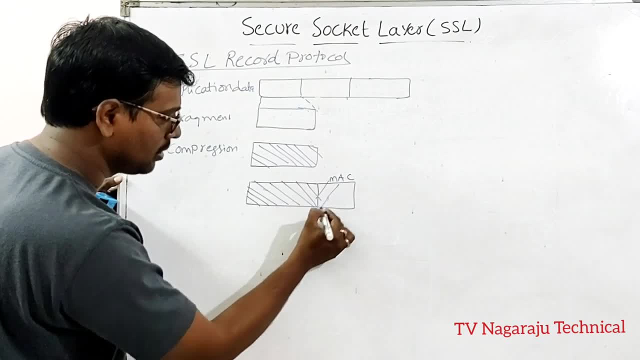 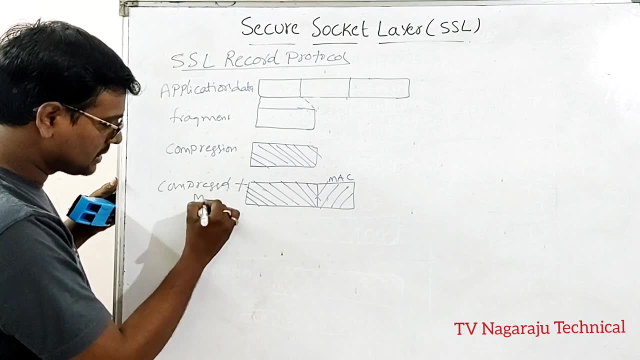 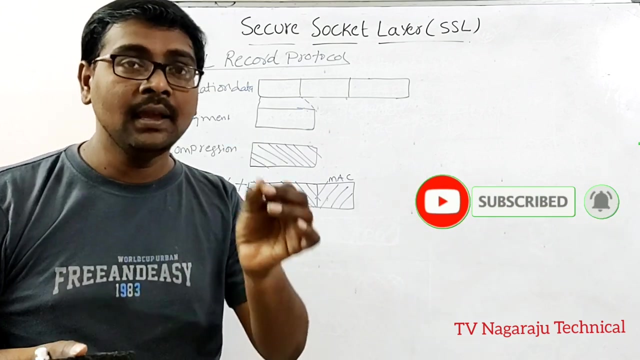 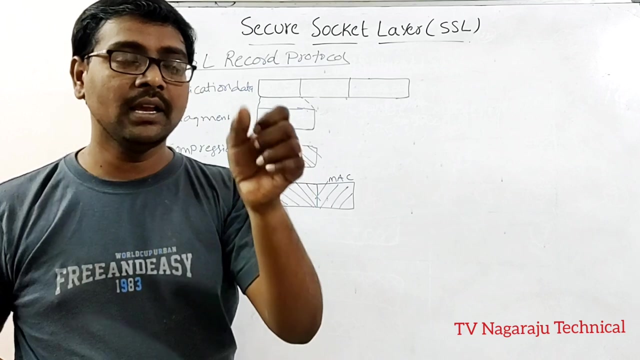 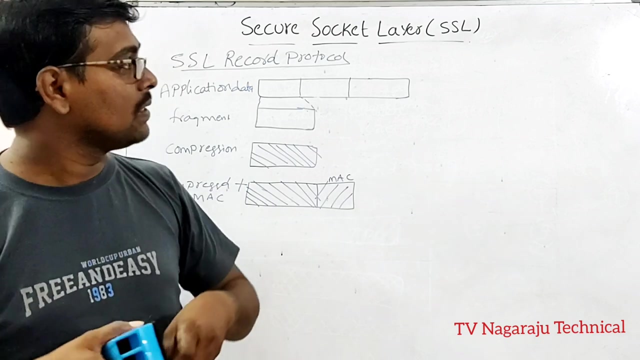 Now you understand the point. Now you understand the point. This my compressor, this is my here. anyway, I will write down compressor plus message authentication code. okay, after this, what is the next step? apply any encryption algorithm. that means you understand. secure socket layer provides the security to the data that is transferred between the client and server. that is. 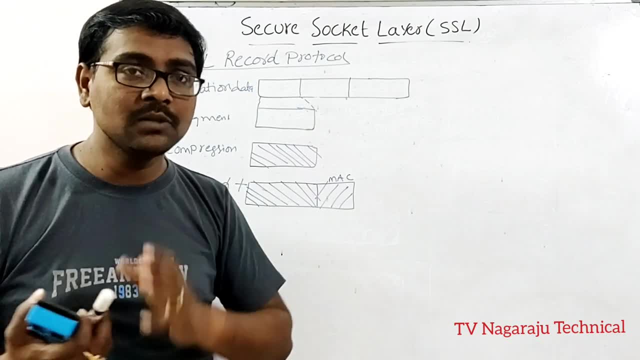 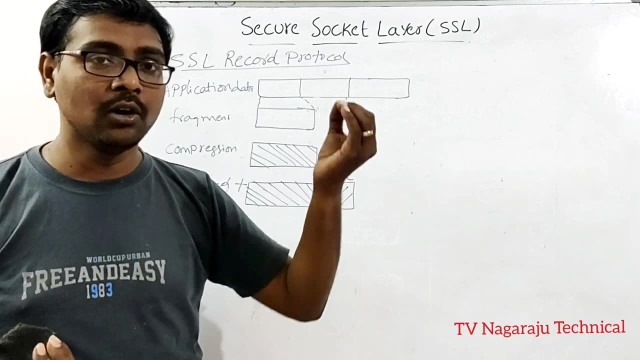 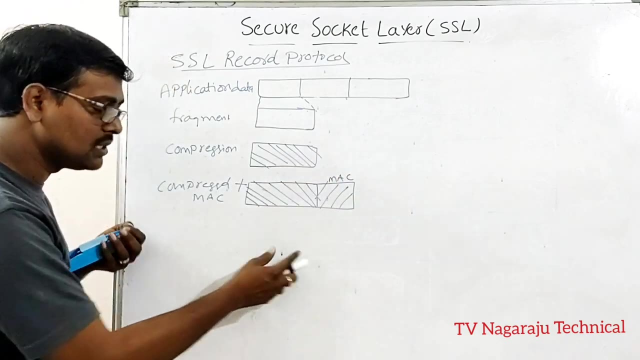 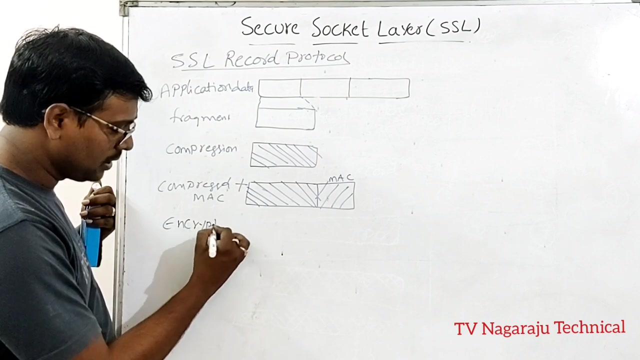 it achieves the confidentiality. what is mean by confidentiality? an injured person is unable to see the data, that is, third party persons are able to watch the data. here I send the data by using encryption. so here this is the procedure I am following. after completion of this one, apply any one of the encryption. 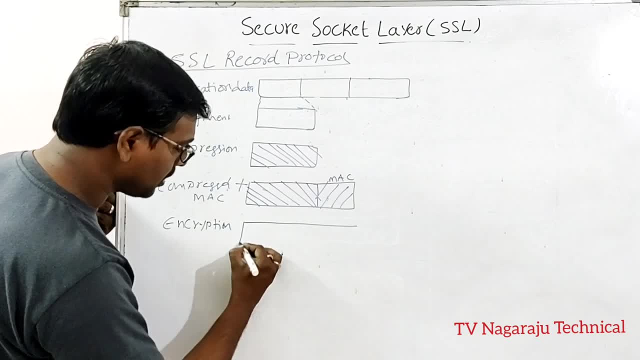 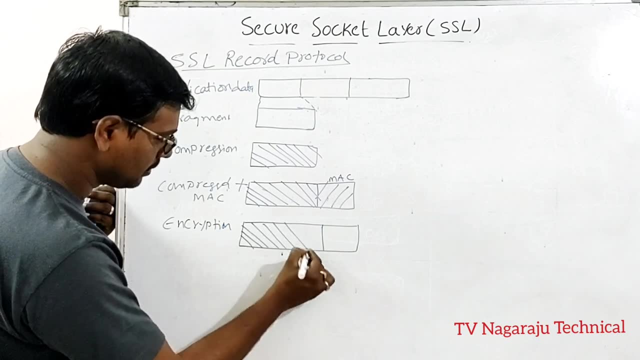 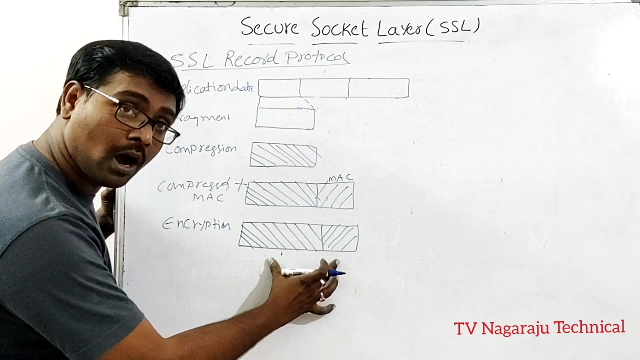 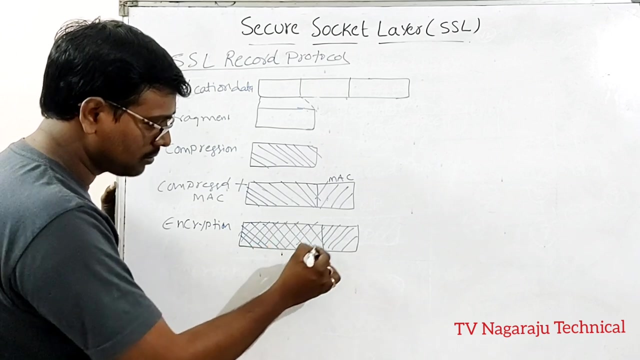 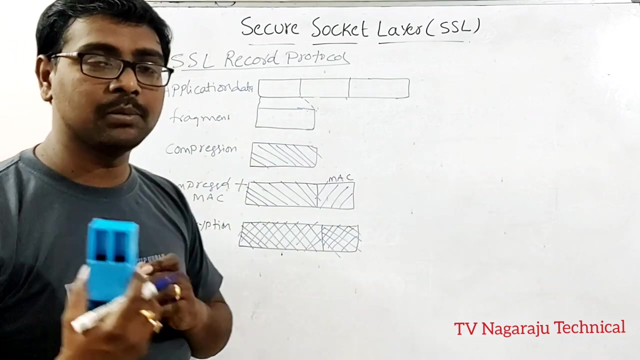 technique. apply any one of the encryption techniques. now this is my compressor data. this is message authentication code. apply the encryption on the entire thing. so on the entire thing. in the sense in this way, apply the encryption now. okay, the everything is completed. encryption is completed successfully. generally. 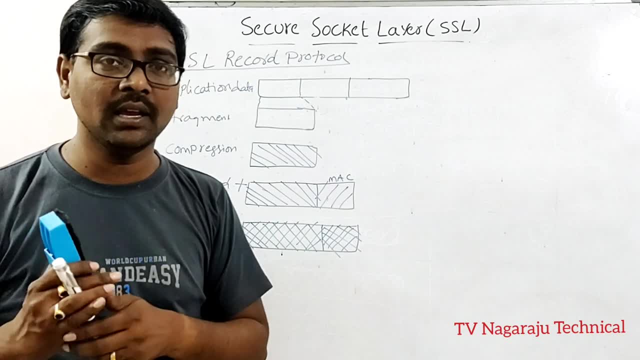 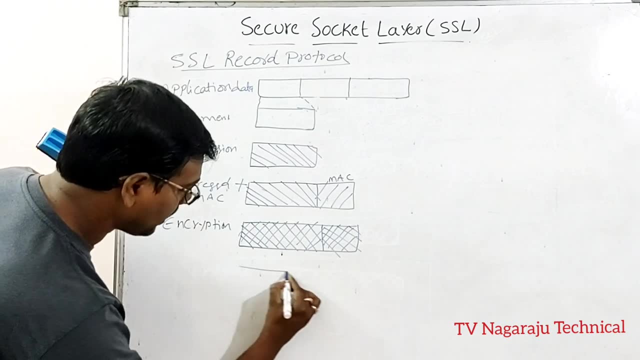 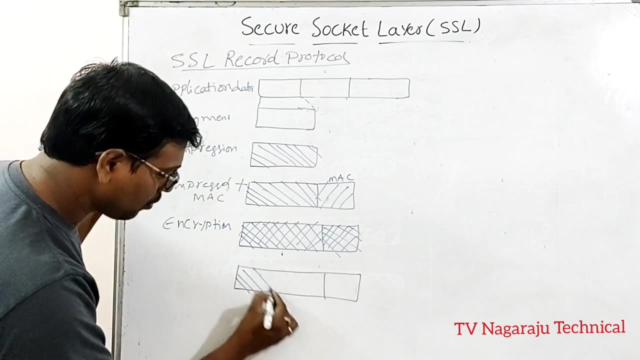 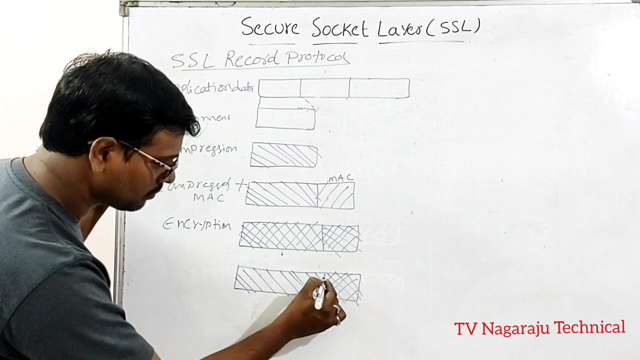 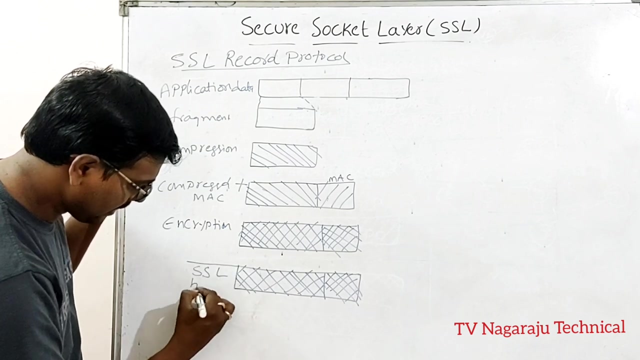 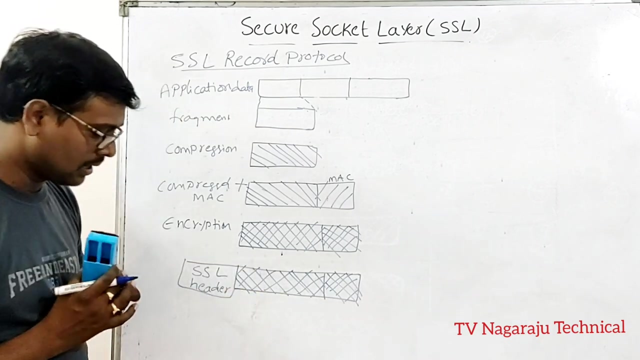 the layers. one layer information is transferred to the other layer in that process. you need to include the headers here also. we are adding one header to the data. after completion, we are adding one header to the data, so that is called a SSL Vi at the SSL HATHER. this is added to the encrypted data. now what? the SSL header? 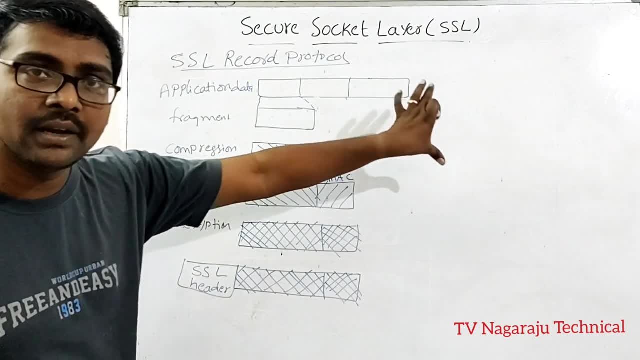 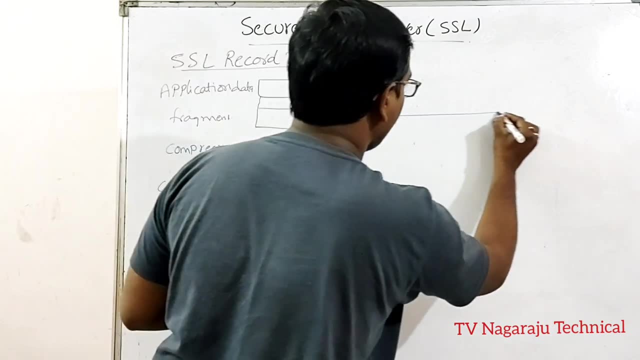 consists of and how that it is represented in a diagrammatic format. remember the SSL header consists of mainly four parts. whatever the SSL HadSON, we are added to the encrypted data, the SSL header and encrypted data, the code. fairly, you can see it is a must-have if you all are using witnessing. 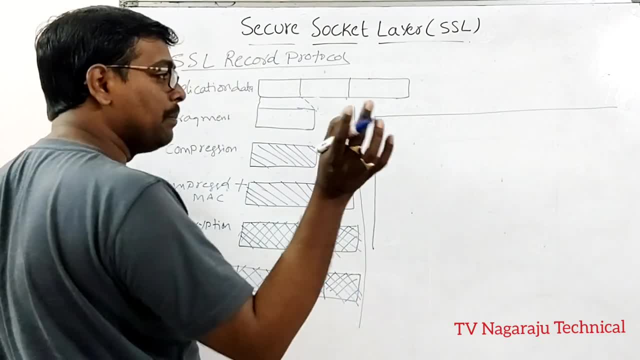 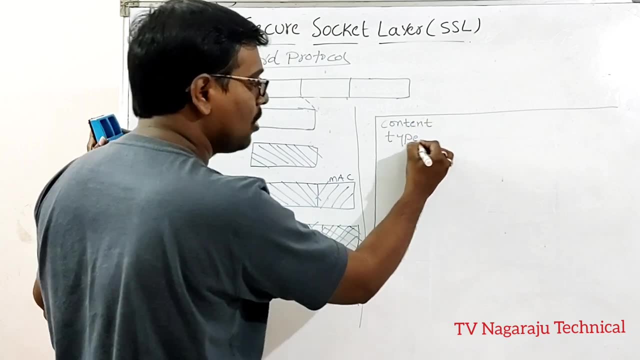 the software if you all are using caption follow often when you have access to a wide range developing source the the edit ���� is there this up to 50 coins but this is quite a shortage but the most often the mainly consists of four parts. The first one is content type. What is the content type? Here 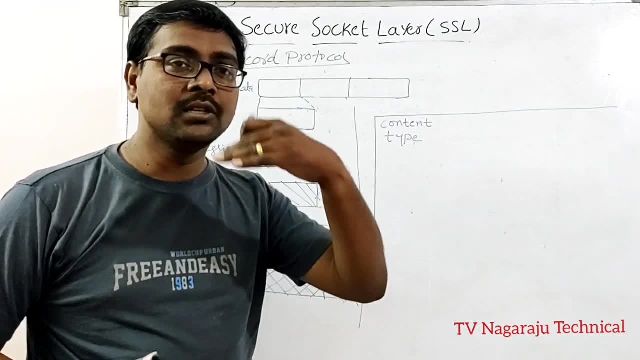 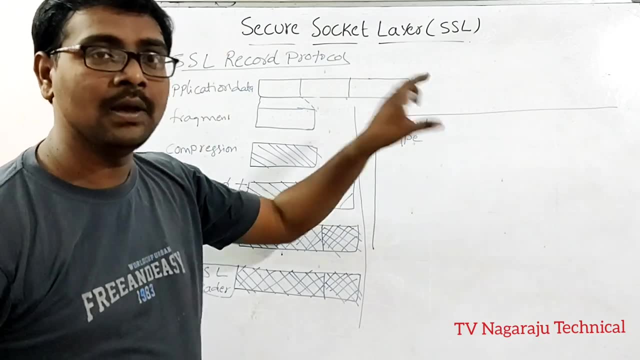 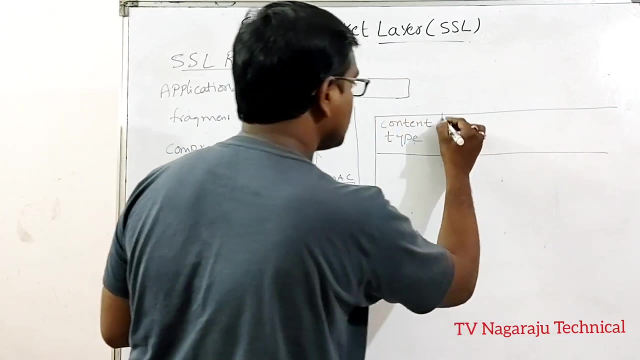 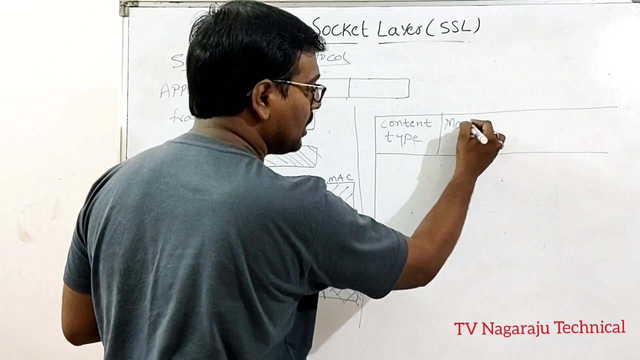 whatever the data that is generated, that is to be processed by higher layer. So to which layer the data is processed. the content type specifies the higher layer that will process the data. Now, second one is we have different versions of SSL, Different versions of SSL. What are the right now? 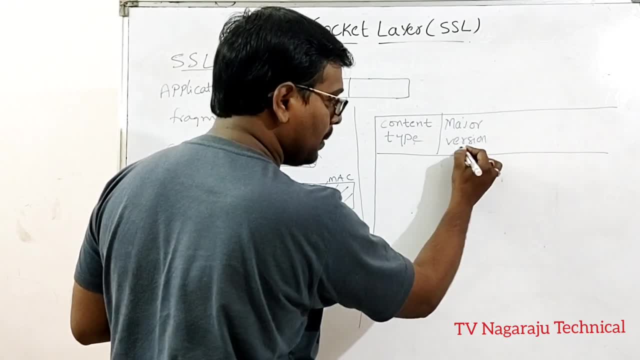 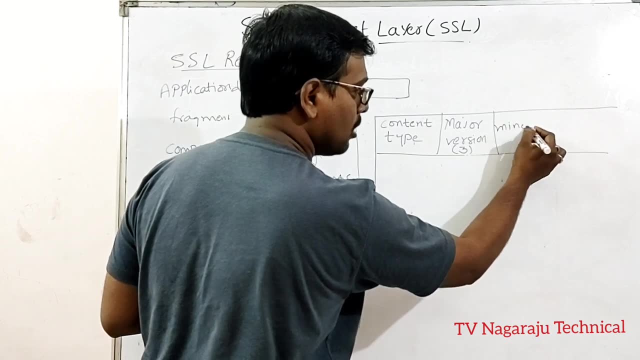 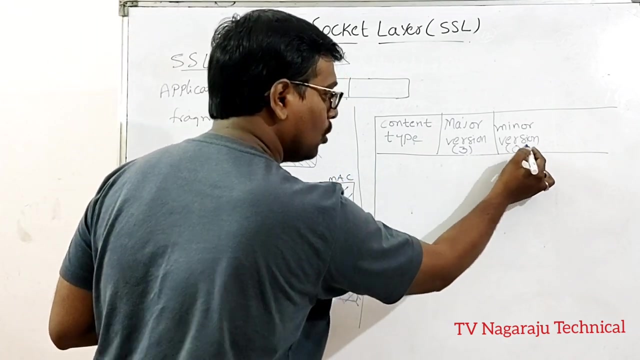 the major version. So right now the major version is version number three. After that the SSL header also consists of minor version. So the minor version is zero. So up to now these are fixed with the major. So the minor version is zero. So up to now these are fixed with the major. So 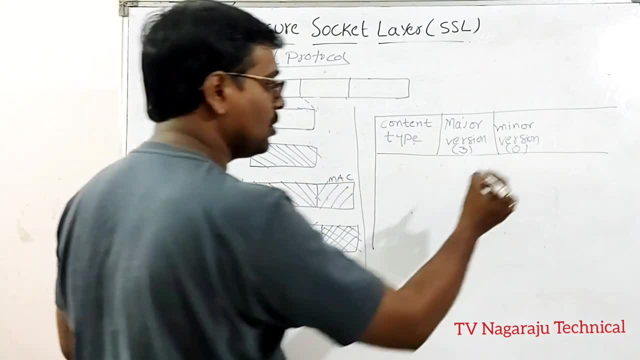 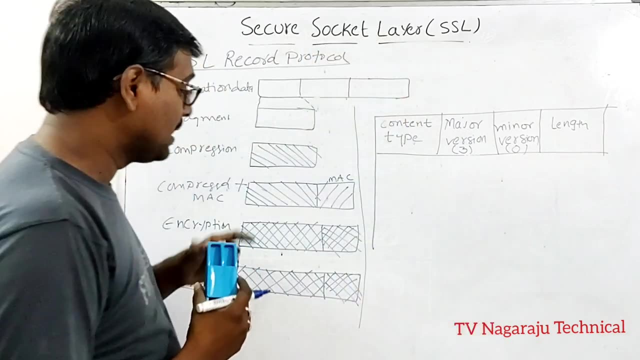 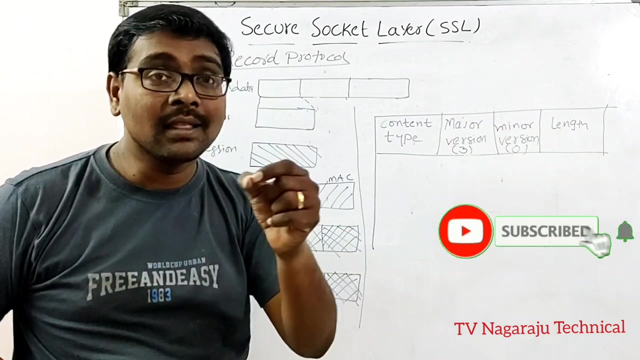 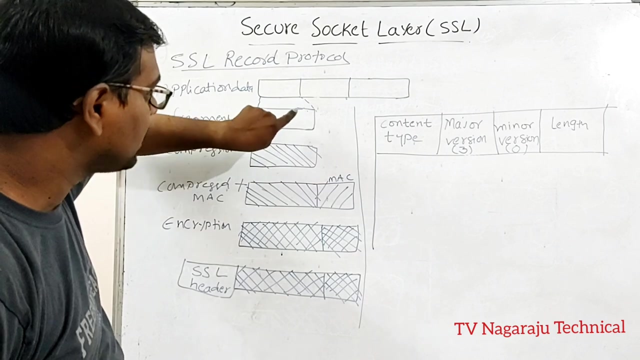 major version is three. Minor version is zero. along with it consists of length. So here length means that if you are performing compression, the length of the compressor data, The length of the compressor data, this one Suppose. if you are not doing any compression, the length of the plain. 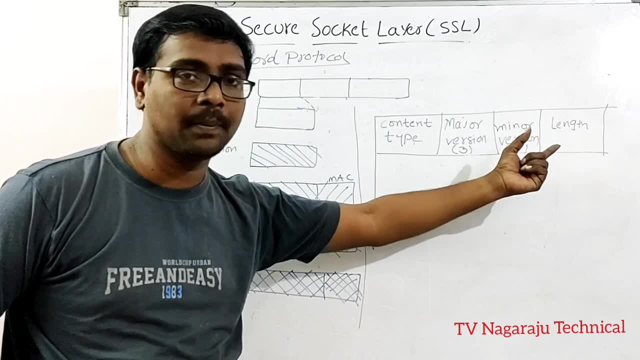 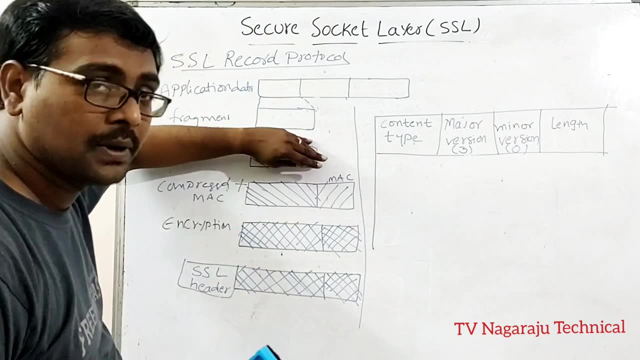 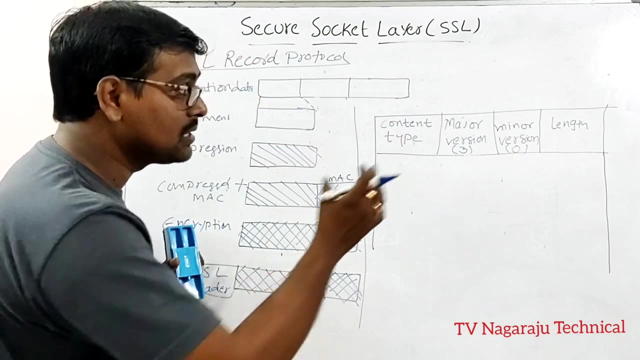 text. That is, compression means length of the compressor data. So if you are not doing any compressor data, if you are not doing, compression means the length of the plain text. I already said that this compression is optional. Okay, Okay, This is the SSL header, Actually, this SSL header here. 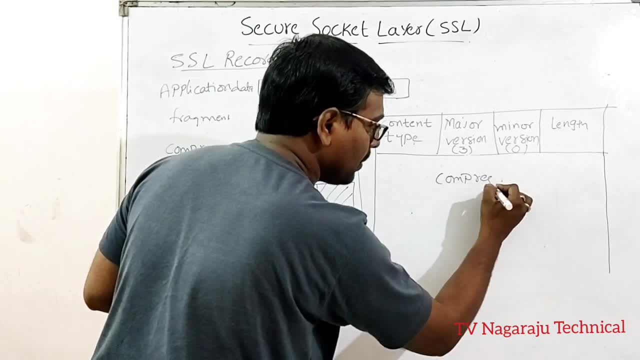 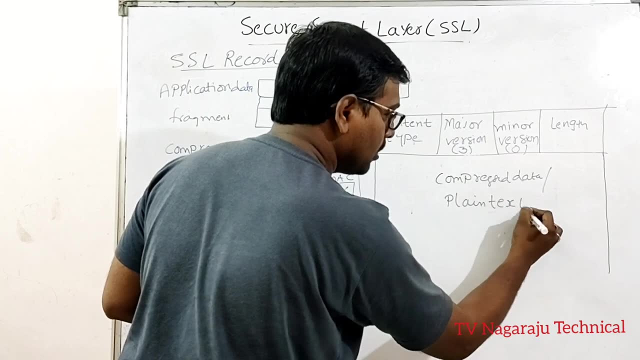 only length. it consists of my compressor data or plain text, Yes or no? So understand the diagram. SSL header: It is the length of the compressor data. So if you are not doing any, compression means the length of the compressor data. So if you are not doing any, compression means the length of the. 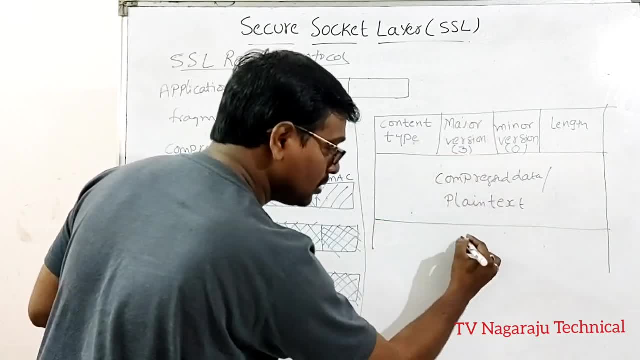 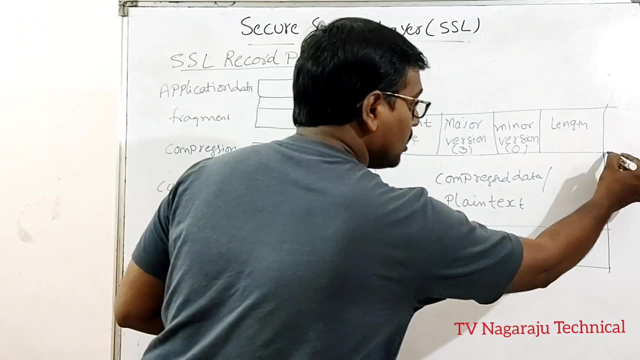 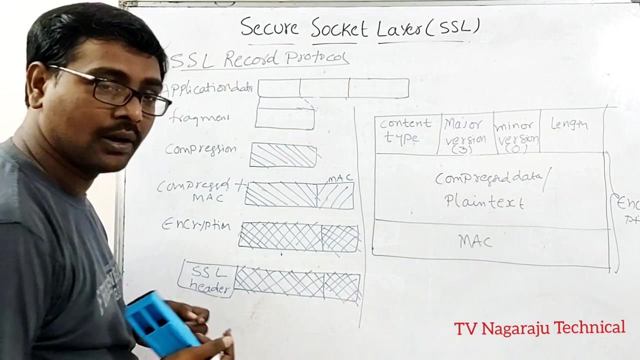 compressor data. So if you are not doing any, compression means the length of the compressor. it is attached to the compression, But it is attached to the MAT Yes or no Message authentication code. Now these two are encrypted. We are performing some encryption. I think now the diagram is clear. 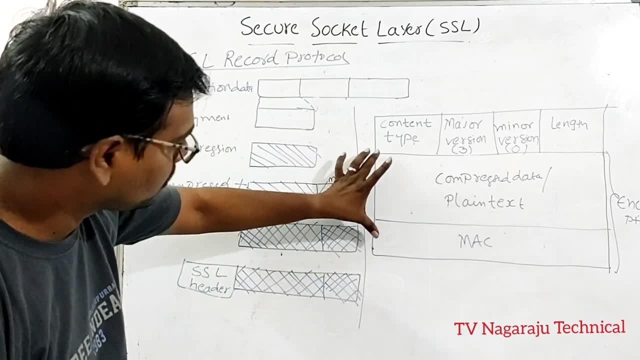 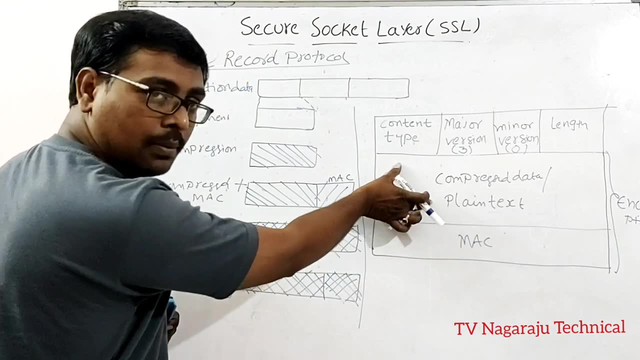 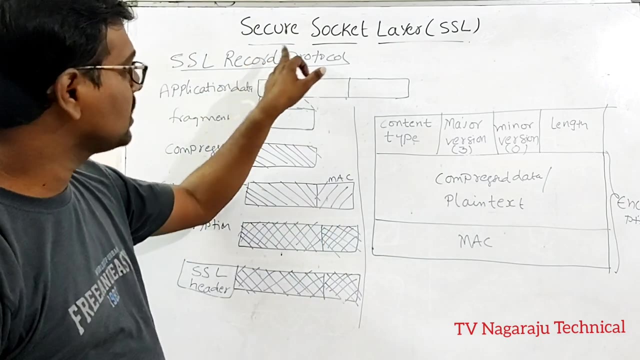 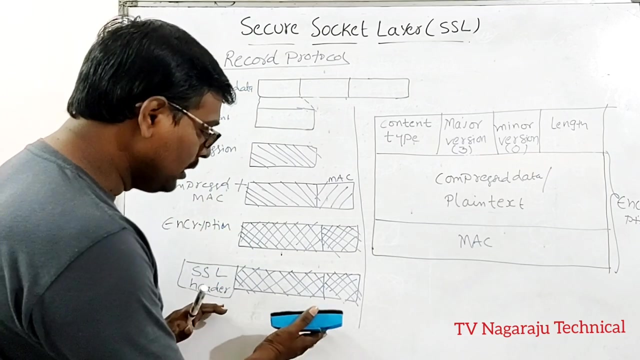 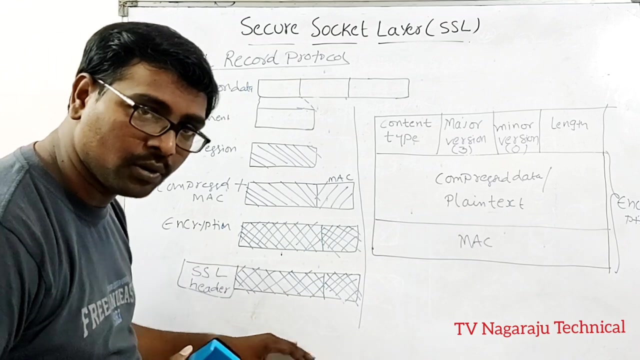 SSL header is added to encryption data. This is encryption. Under this encryption, the first part is compression data plane test. the second part is message authentication code. so this is the SSL record protocol. SSL record protocol- okay now, even though it generates the output, remember one point: the SSL record protocol generates some output. this: 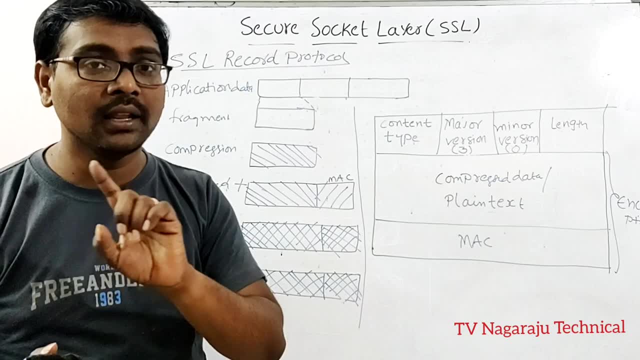 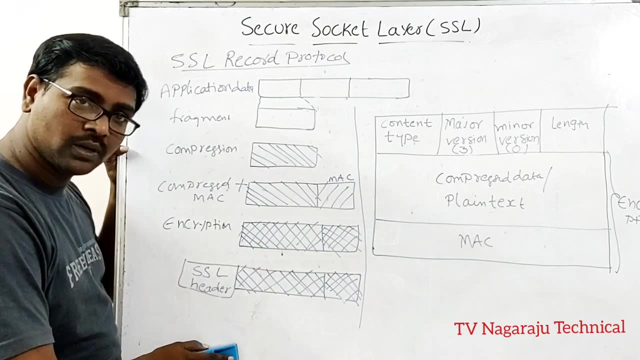 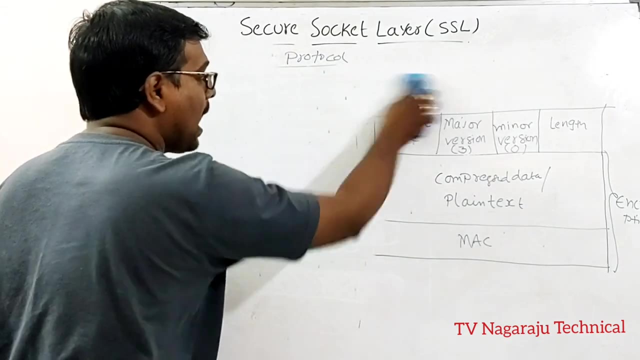 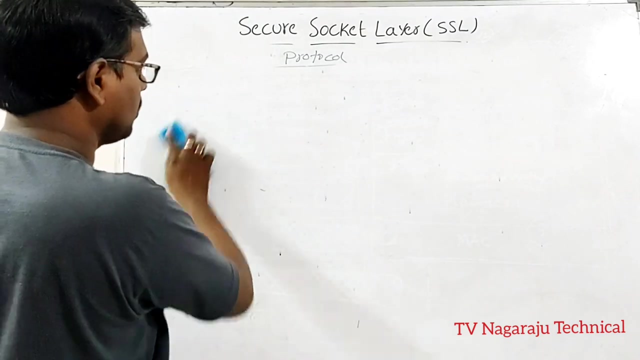 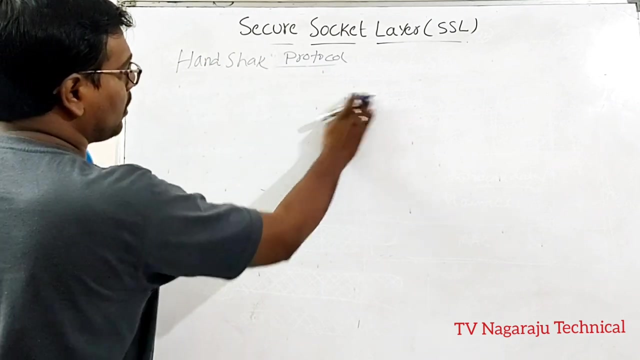 output is in pending state, not in current state. what is this one? I will explain after completion of second protocol. I think the first one is clear: yes, move to the second protocol, that is, handshake protocol. the second one is handshake protocol, handshake protocol, the protocol, the handshake protocol, the. 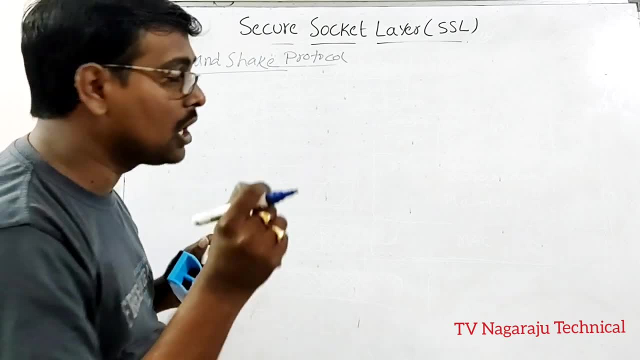 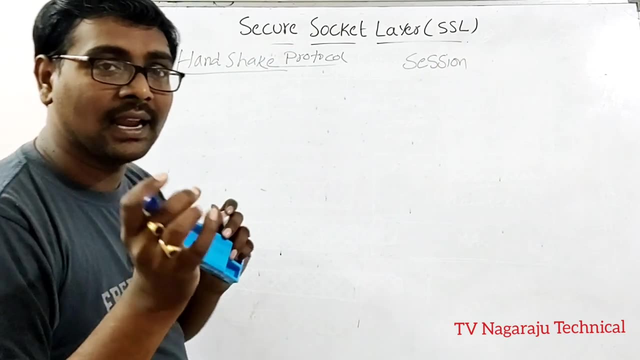 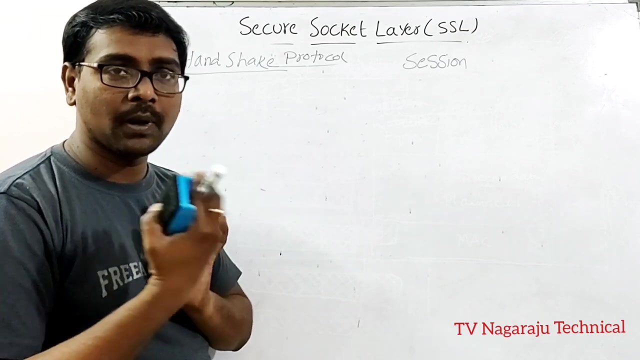 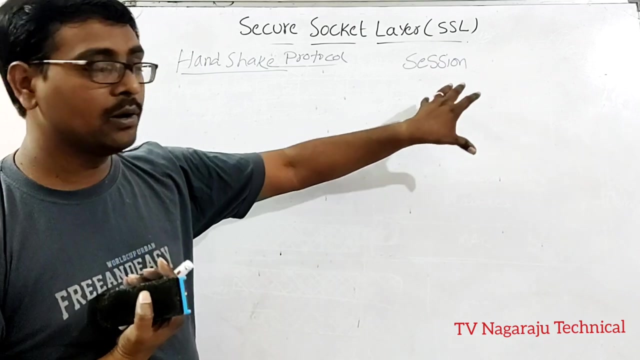 protocol, the handshake protocol. the main purpose is used to establish a session. used to establish a session among the client and server. I think you know the meaning of session. so session means, suppose you are performing some operation. you are performing, suppose income tax department. whenever you are open some income tax department, it opens. 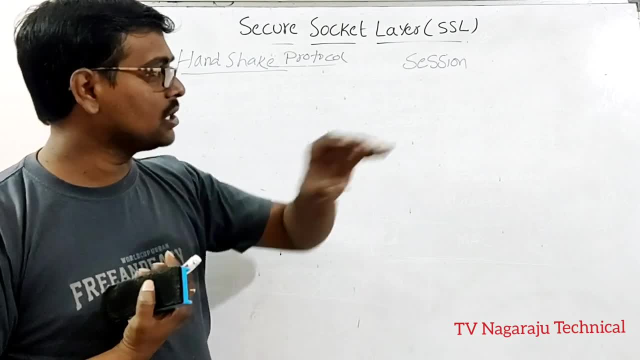 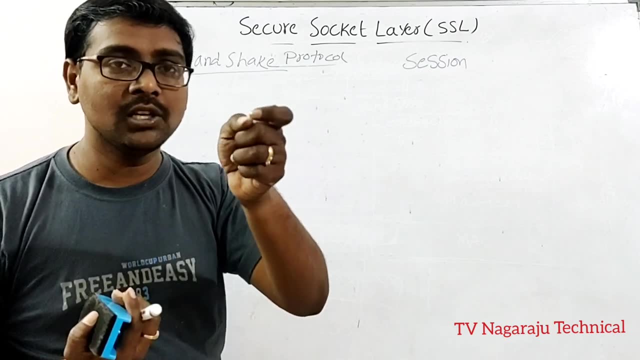 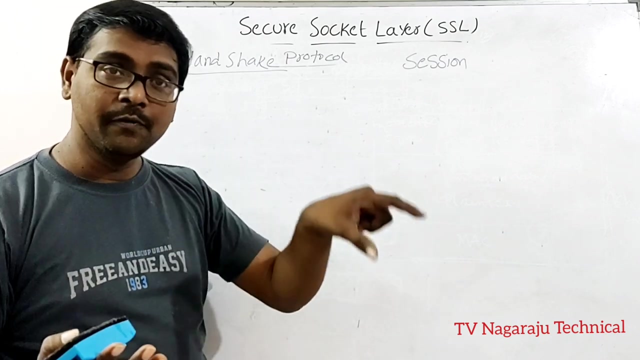 a session of 10 minutes or you are at a bank application, it opens a session of 5 to 10 minutes, so that means it establish a session. each and every operation need to be performed within that session. suppose: if you are ideal for these 10 minutes, the session closed. if you are active, again the session. 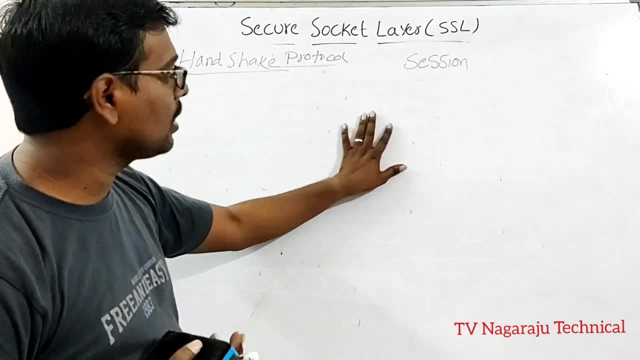 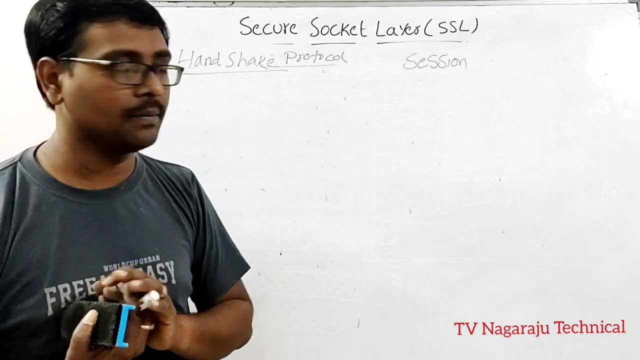 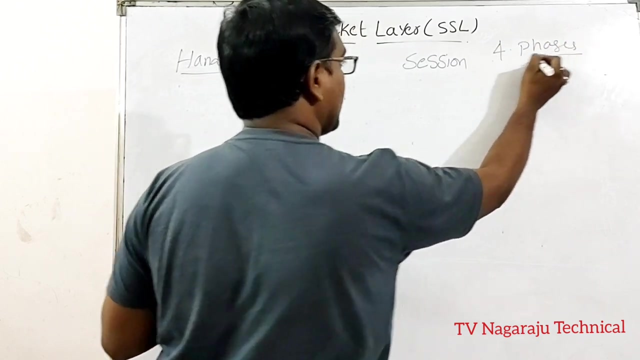 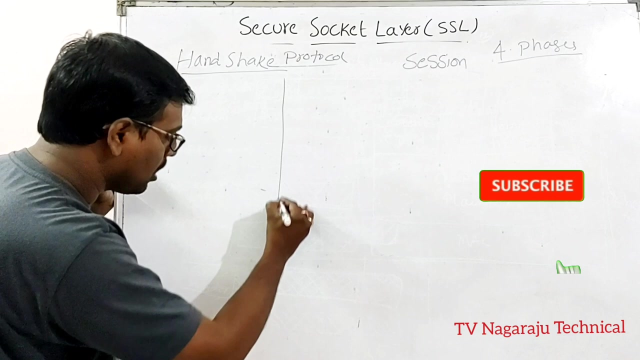 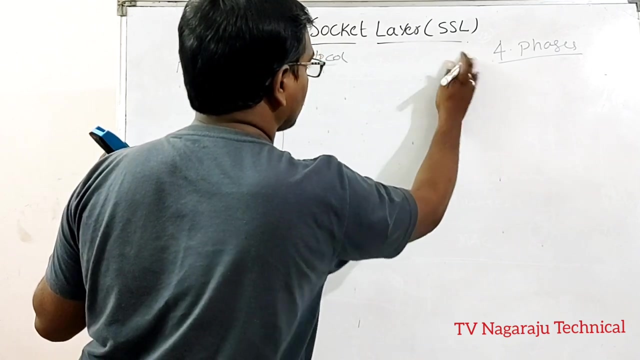 reestablish. now this handshake protocol is mainly used to establish the session between the client and server. now this protocol is completed in four phases. the handshake protocol is completed in four phases. I will explain each and everyone. assume it is the client, this is client and here server client. to end, 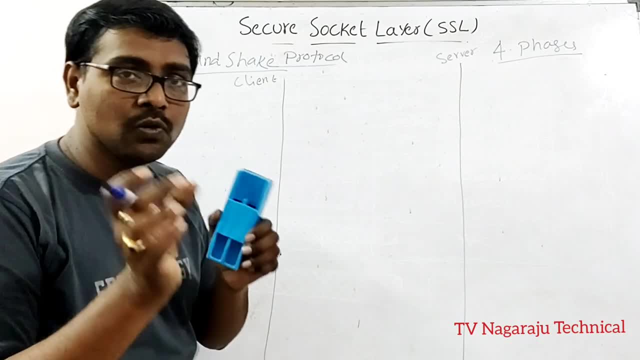 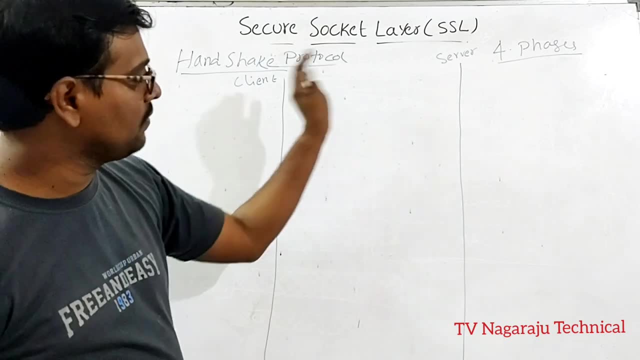 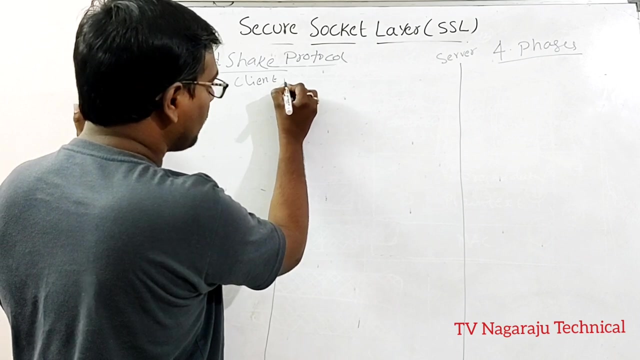 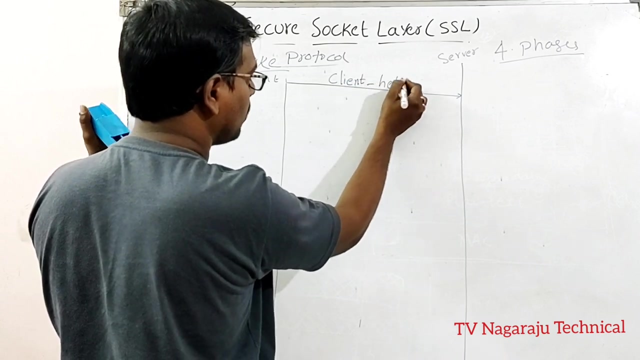 server. follow, step by step, the first two phases among the four phases. the first two phases is establish the connection. even though the session is created within the session, you need to establish the connection for that. what happened? client to some? send some message? client hello, client hello is the message sent by the 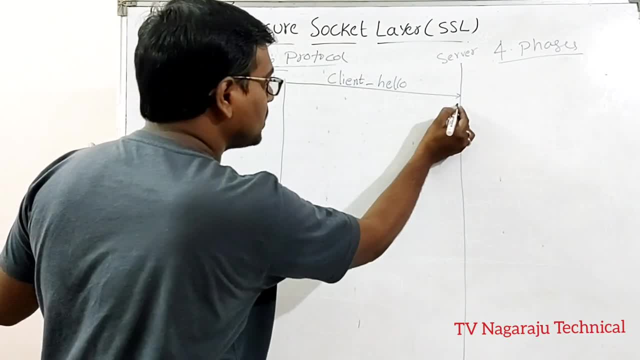 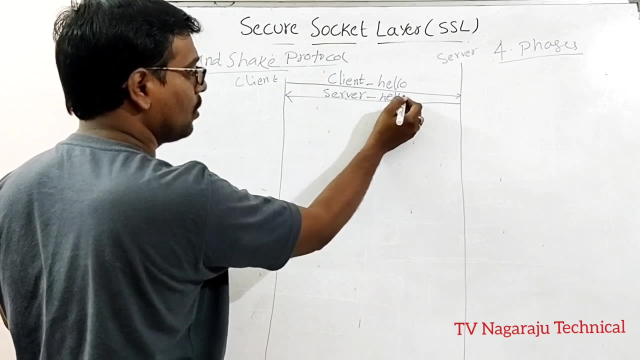 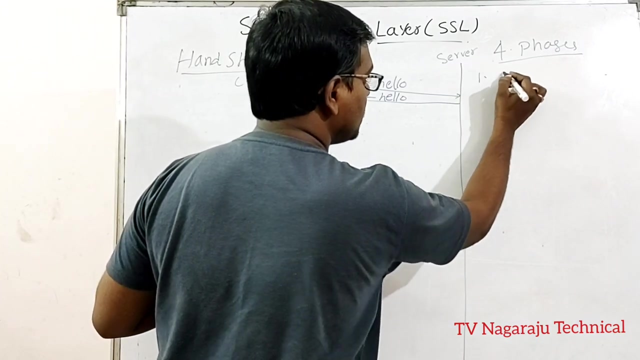 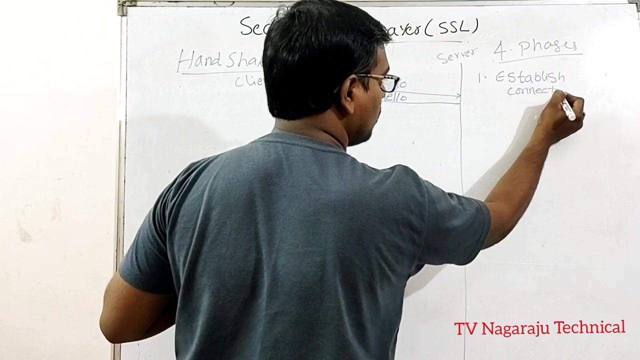 client to the server. on receiving the message, server also sends the message. server has to send the message to the server. server has to send the message to: hello. okay, by transforming these two messages, my first two phases completed. this is phase one. the phase one is establish a connection, yes or no, by 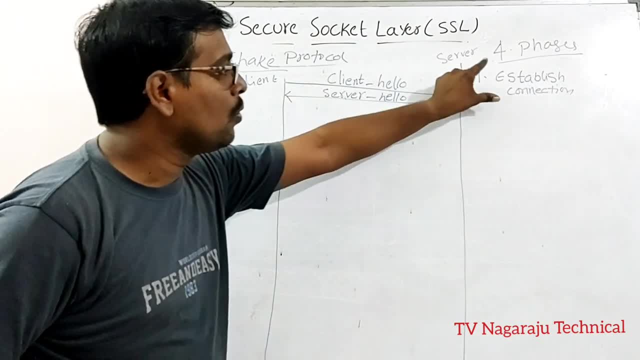 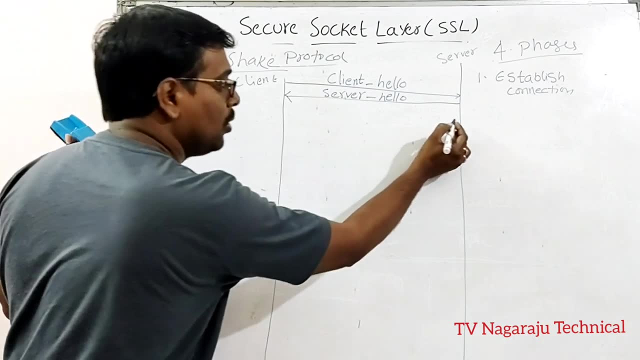 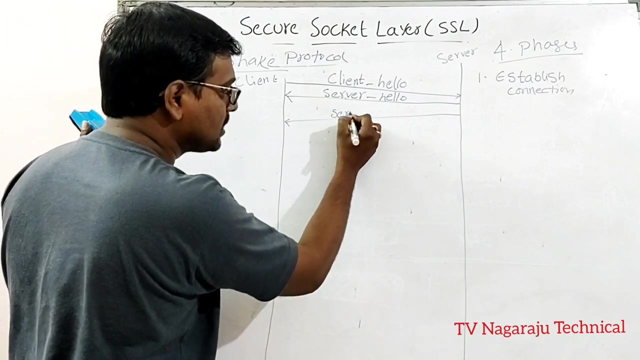 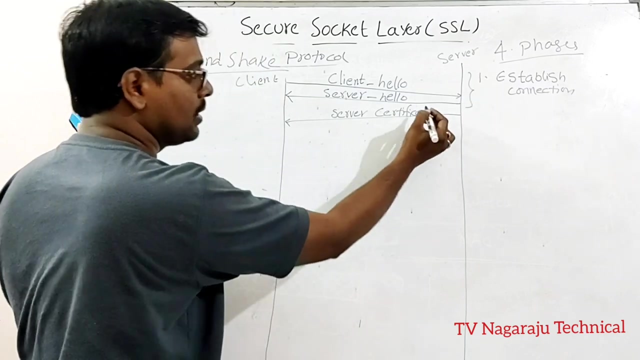 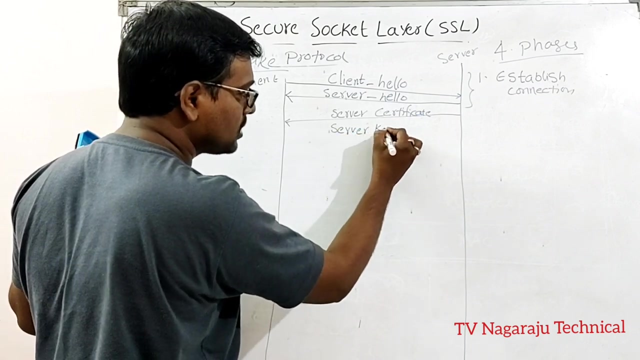 transferring the client hello and server hello. we are establishing a connection. okay, after completion of phase one. now the server sends some information. what are the information? what about the information server certificate? this is server certificate. this is phase one, so the server sends server certificate. the server also sends server key exchange. server key exchange. 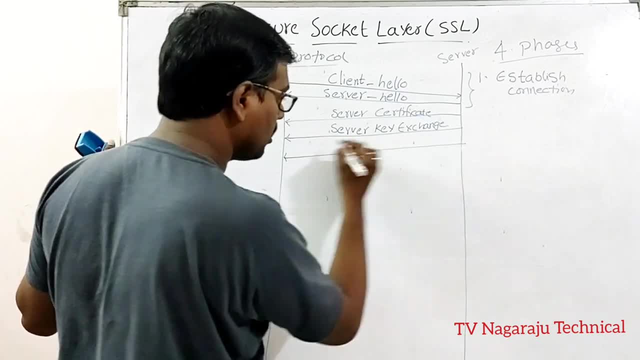 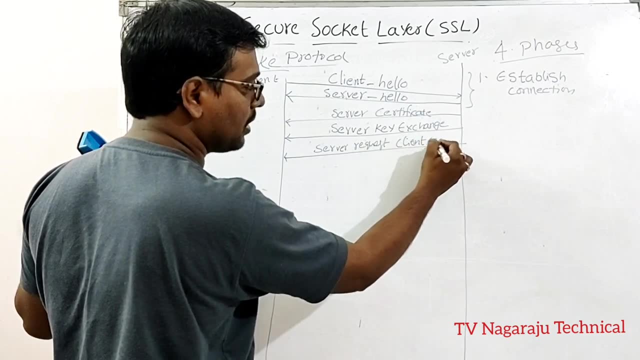 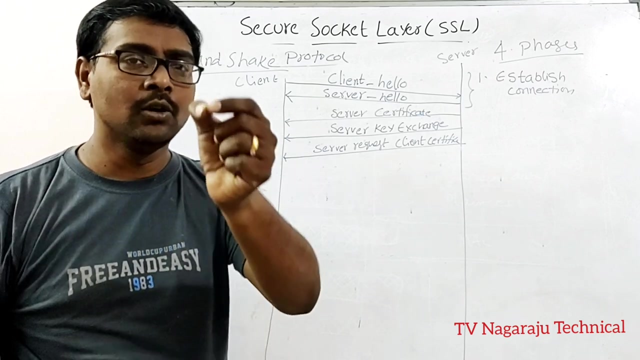 this is the second one- and the server also requests request рын그. Server request the client certificate. Okay, Server sends their own certificate. What is mean by certificate? You know thing? Anyway, by the end I will explain the concept of certificate. 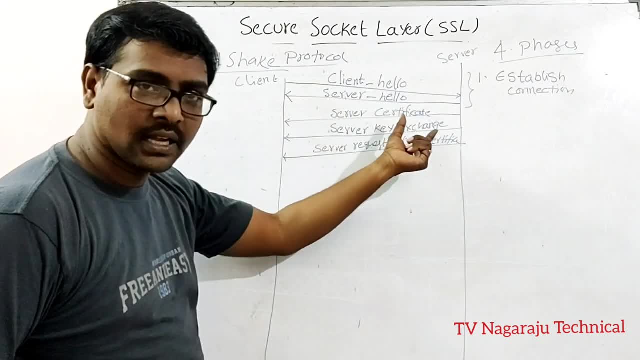 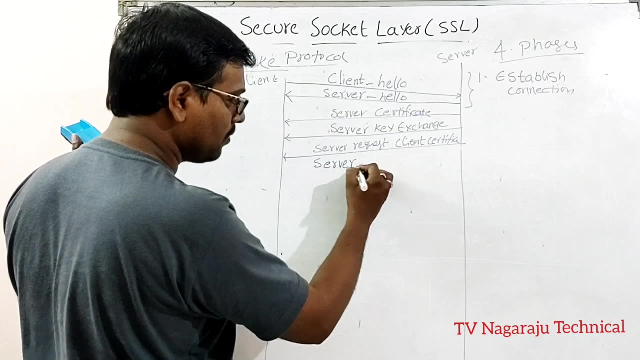 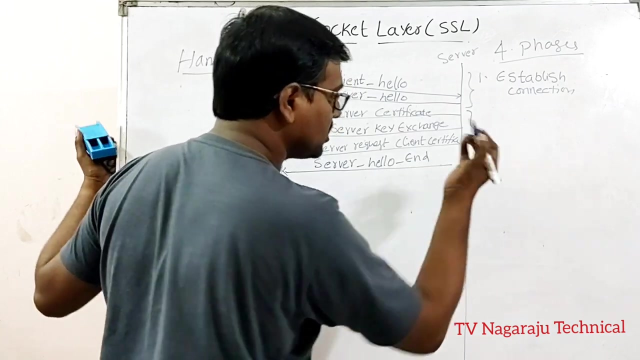 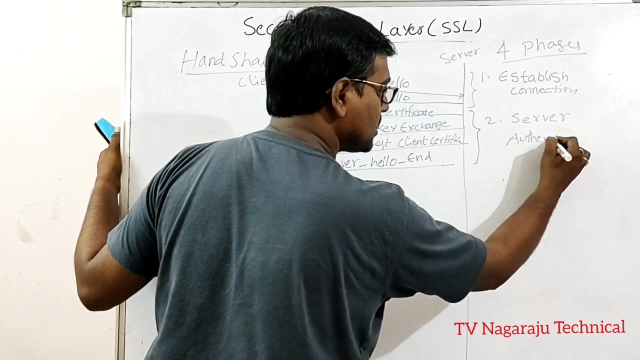 Server send their own certificate And server sends a key exchange And request for the client certificate And finally, server hello. end So by sending this statement. this is phase 2.. The phase 2 is simply server authentication, Yes or no. The server sends all those information. 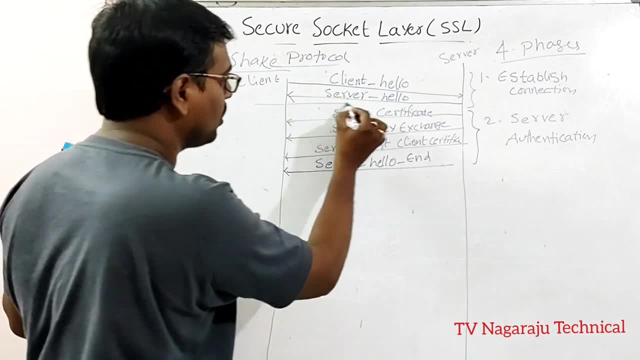 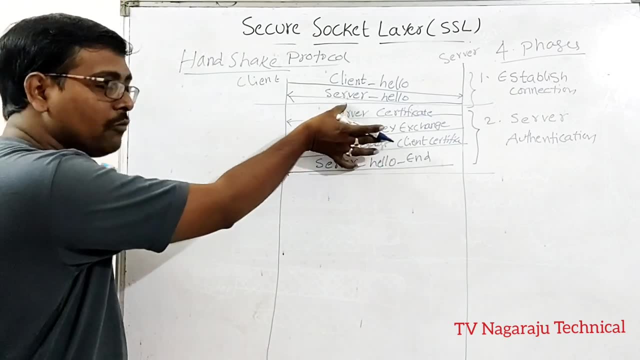 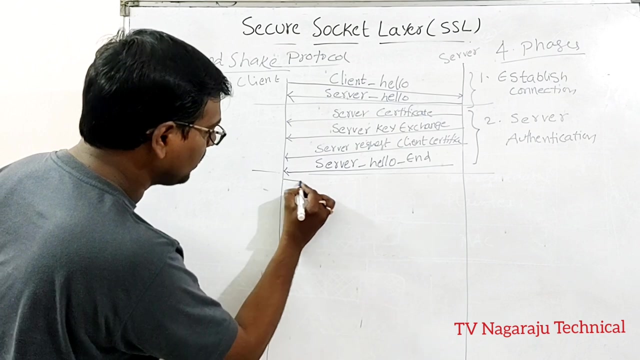 That is called server authentication. Now here up to phase 1.. Phase 2. Coming to phase 3.. Exactly, Once these things are received by the client, Client authentication need to be done. Now, what the client do? Same sense. 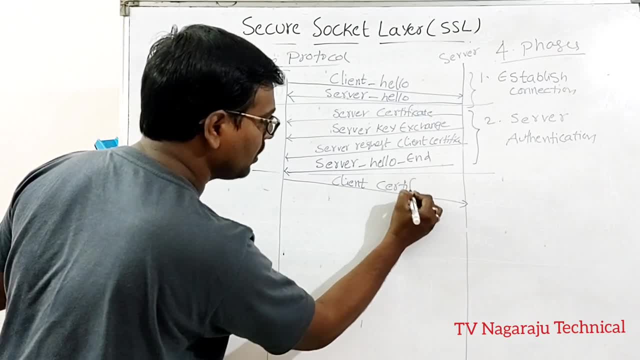 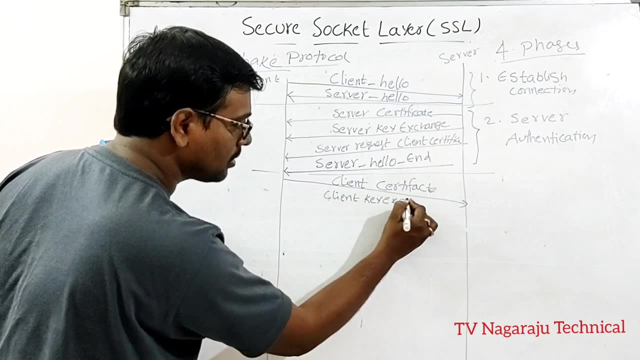 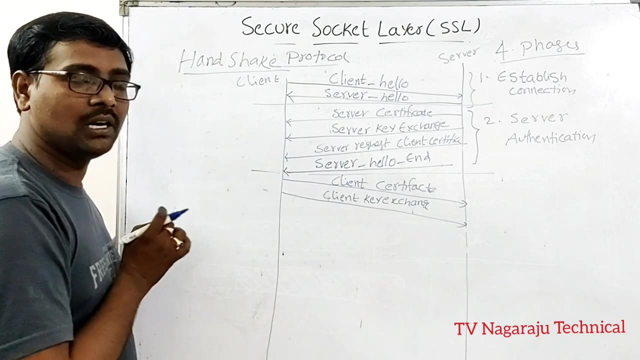 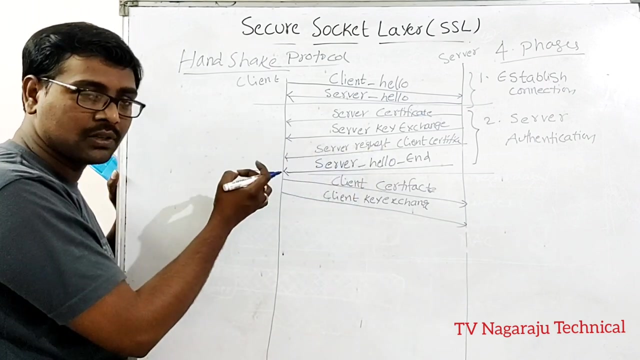 Client specifies Client certificate is transferred to the server And client key exchange. Whatever the information received from the server, Exactly the same information, But it is related to client key exchange And the request is not at all required. Why? Because already I got the server certificate. 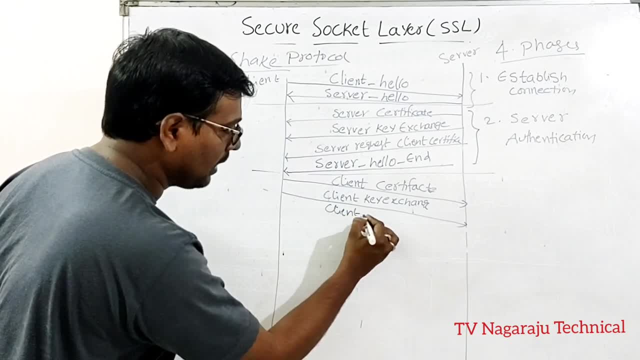 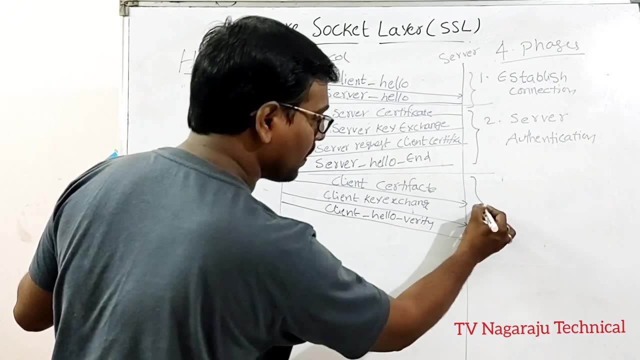 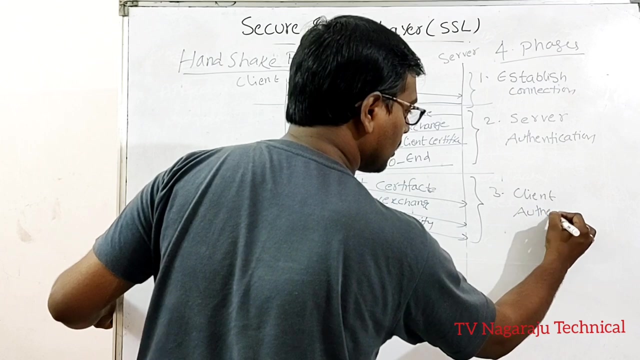 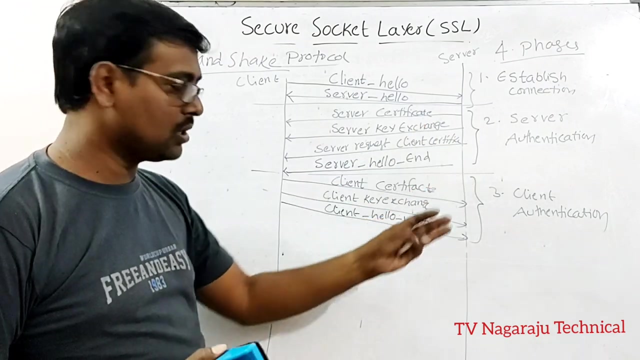 I am sending the client Now. client hello verify. Client hello verify is transferred. That means the third phase is simply client authentication. The third phase is client authentication. Now the server and client are authenticated each other In between. they transfer different messages. 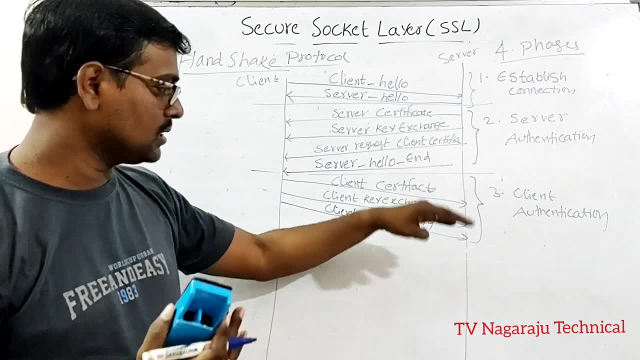 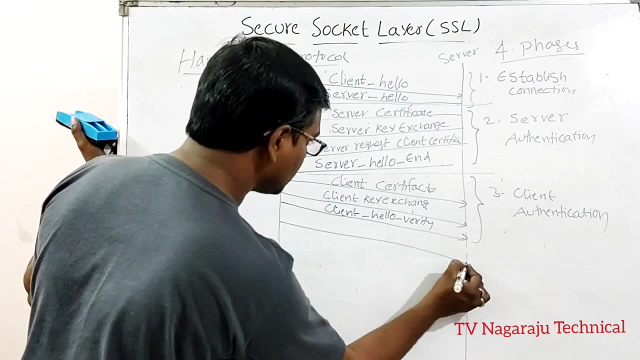 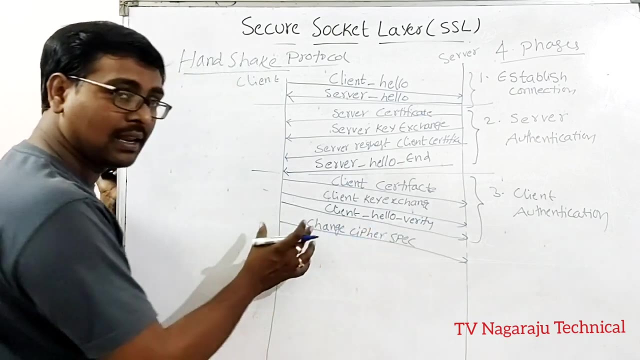 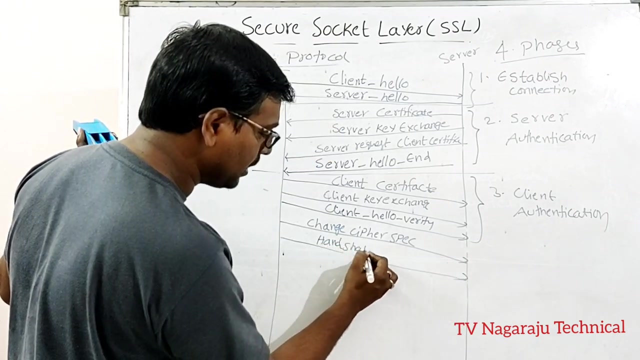 Once the authentication is completed, different messages. After completion of all the messages, you have to stop Yes or no For this. client send change cipher spec protocol, Client sends change cipher spec protocol And the client send handshake completed, Handshake completed. That is from the client side. 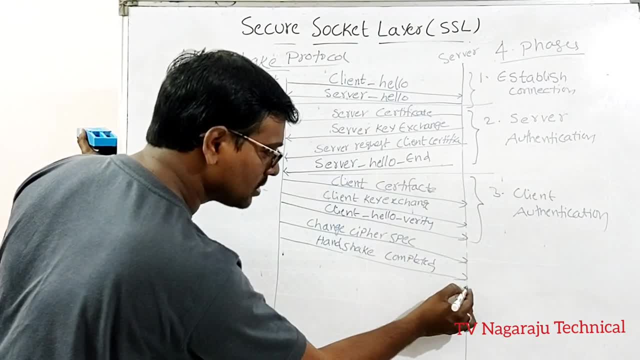 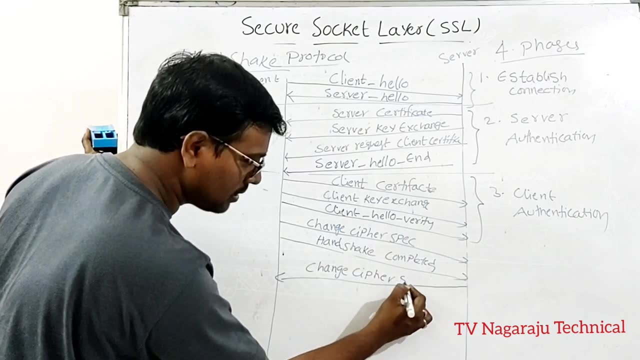 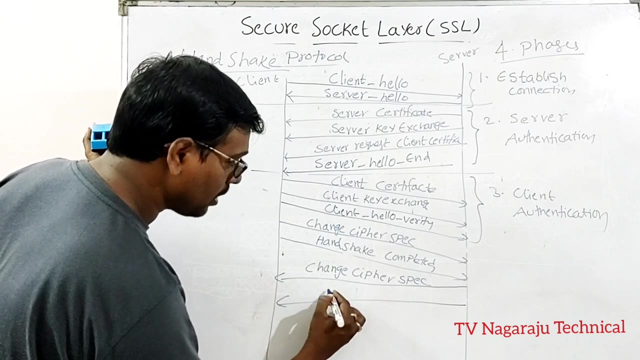 That is, The server is ended. Similarly, on receiving this one Server, also do this one. What is this change? cipher spec. I will explain. This is my third protocol, Yes or no? The protocol stack. This is third protocol. And then server also send handshake completed. 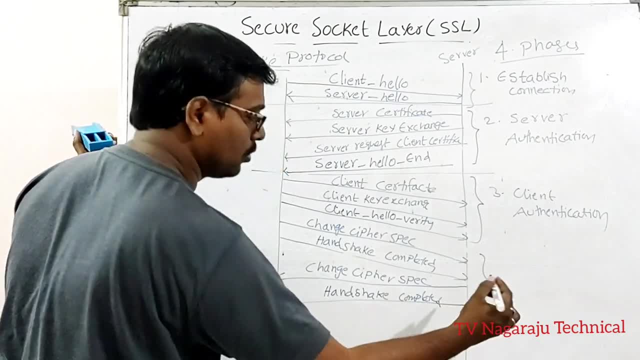 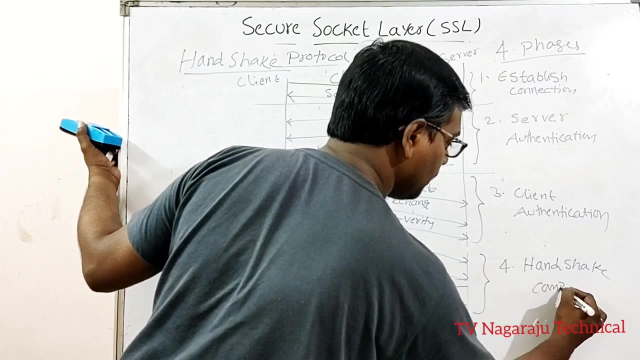 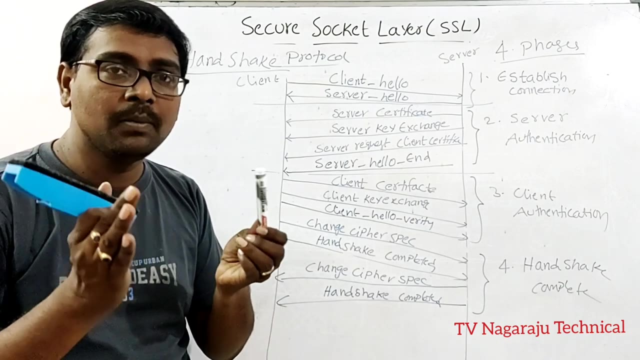 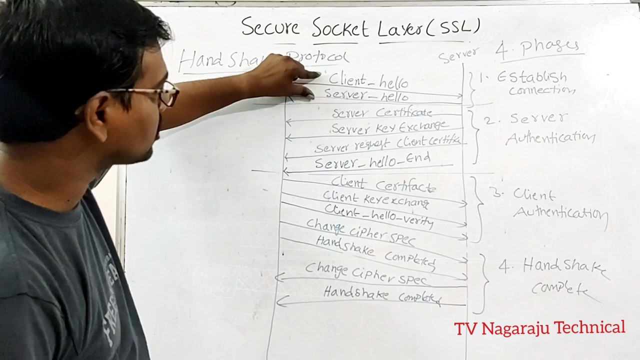 Handshake completed. This is the fourth phase. What is the fourth phase? The fourth phase is completed. Completion of handshake. Completion of handshake. So this is handshake protocol. The main purpose is establish a session between the client and server During the session. the first two phases. it establish the connection by transferring the hello messages. 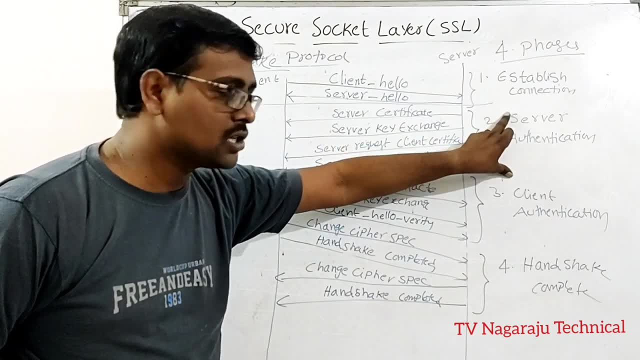 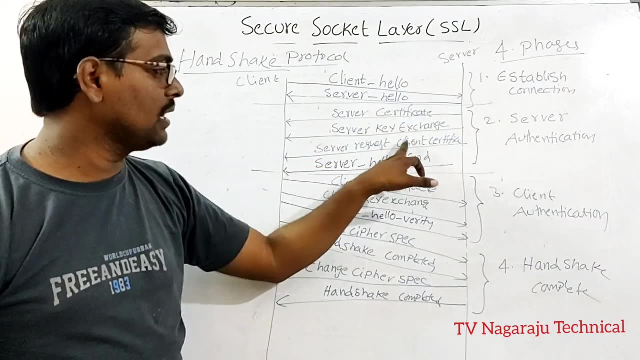 Now you need to verify the authentication of the server By sending the server certificate along with key exchange And it request for the client certificate. Similarly, you need to prove the client authentication. The client send the certificate along with key exchange If, once it is completed, 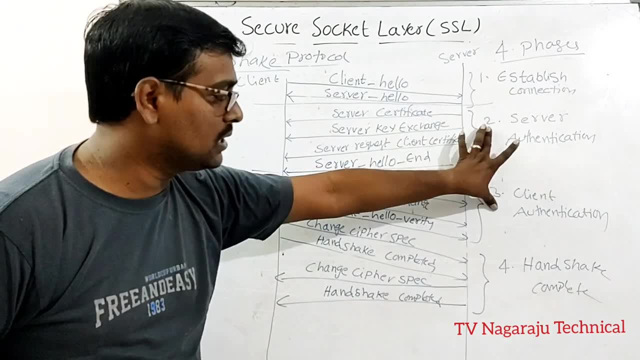 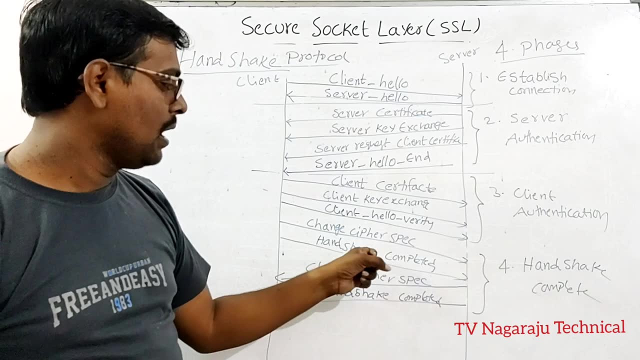 Change. cipher spec protocol is called. Why you are calling this one. I will explain. After calling this one, The handshake is completed. Similarly, from the server side also, the handshake is completed. Now, among all these things, You need to know this important thing. 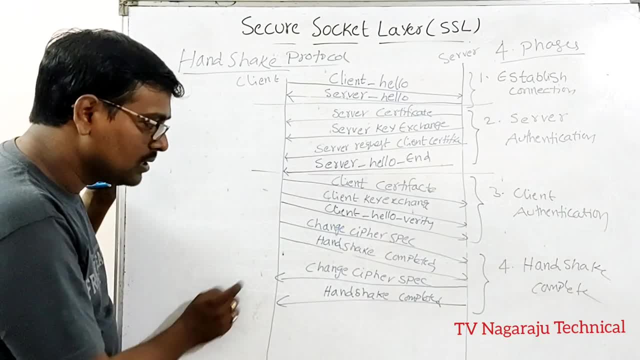 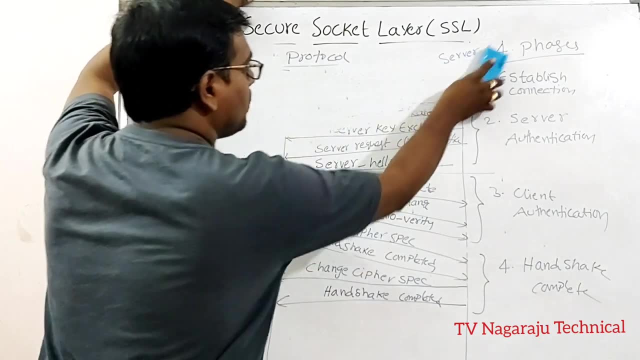 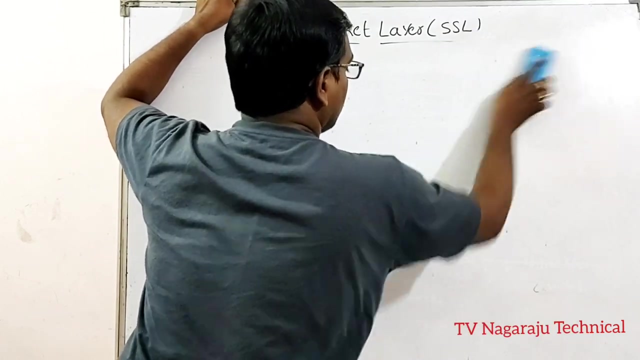 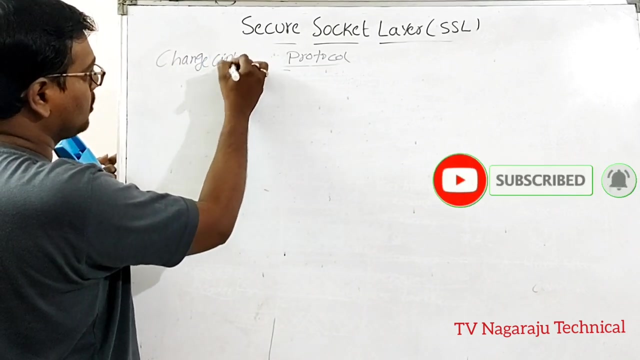 You need to know this important thing, That is, You need to know this important one: Change cipher spec protocol. I will explain This change cipher spec protocol. This change cipher spec protocol. This change cipher spec protocol. Change change: change cipher specification protocol. 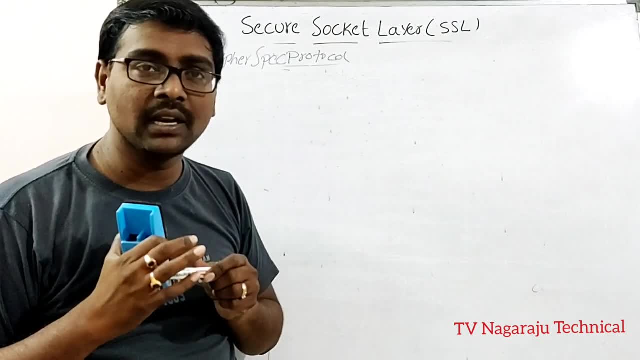 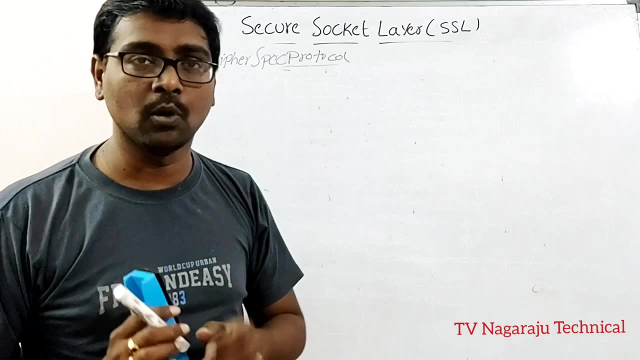 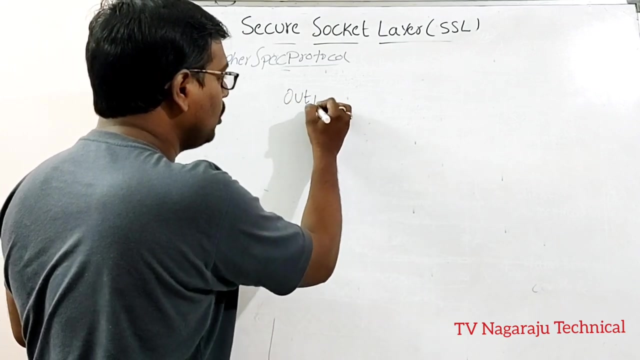 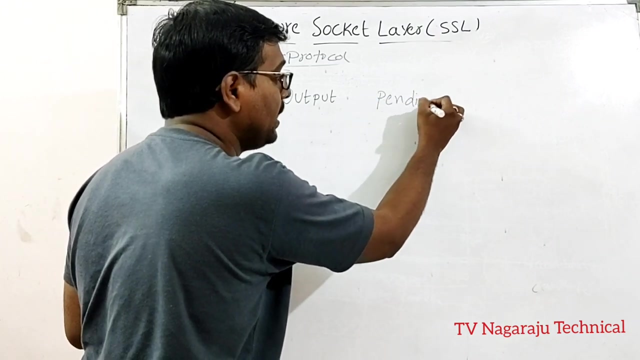 Now first SSL record protocol. Now first SSL record protocol. Now first SSL record protocol automatically generates some output. Remember one point: Until the completion of handshake protocol, Until the completion of handshake protocol, The output generated by SSL record protocol is in pending state. 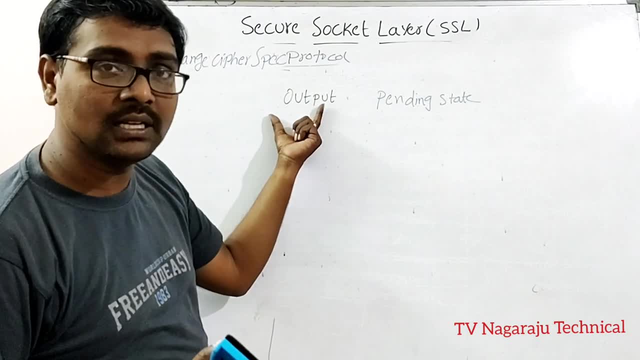 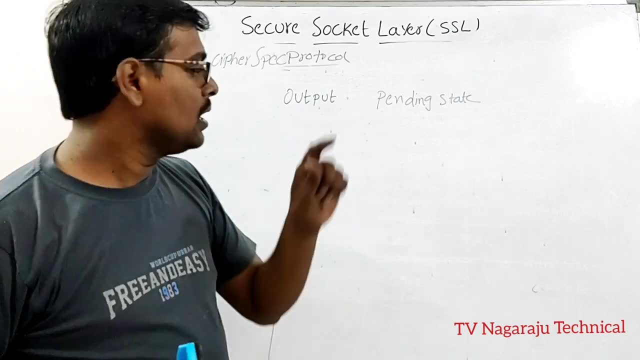 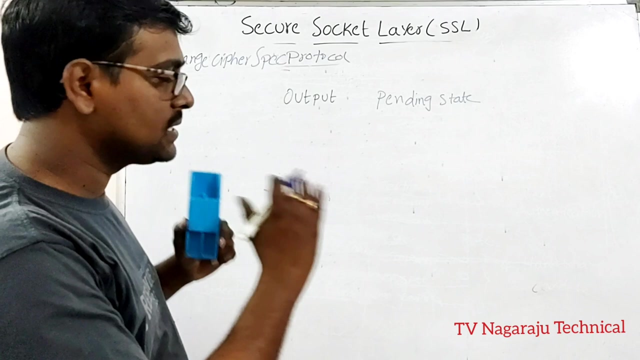 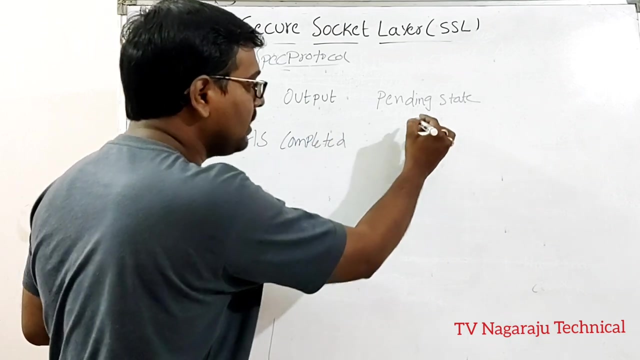 Remember the point. Again, I am repeating: SSL record protocol generates some output. now, until the completion of handshake protocol, the output generated by the ssl record protocol is in pending state. once the handshake protocol, once the handshake protocol completed, then the output in the pending state is copied into current state. 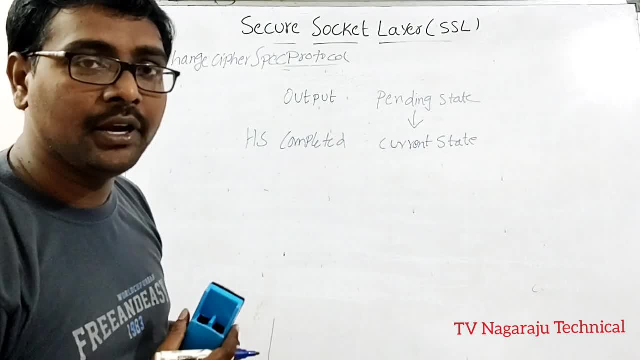 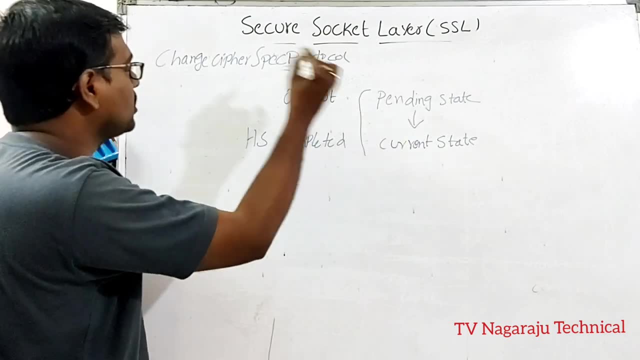 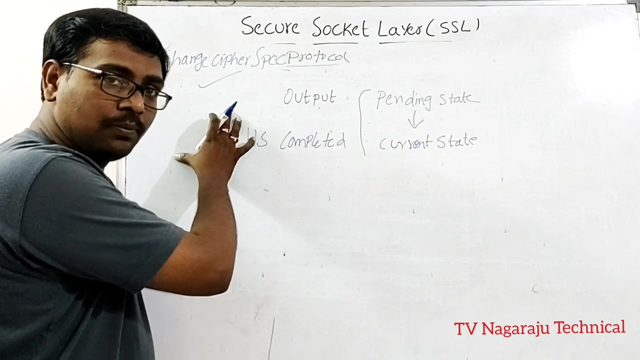 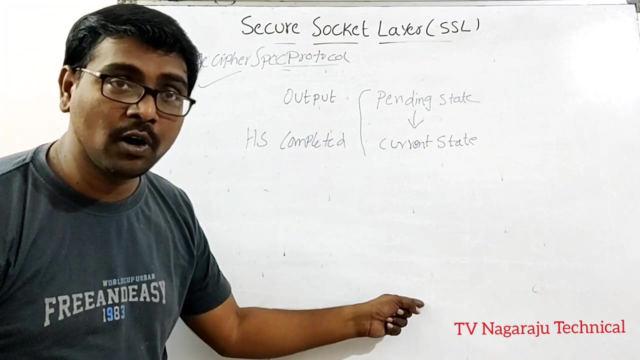 the output in the pending state is copied into current state. you got it now. this conversion of pending state into current state is done by change cipher spec protocol. now you understand. so whatever the output generated by the ssl is in the pending state once the handshake is completed. you observe, in the last two point of handshake i am using this. 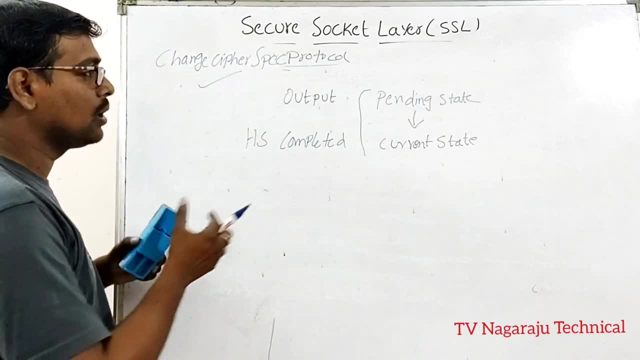 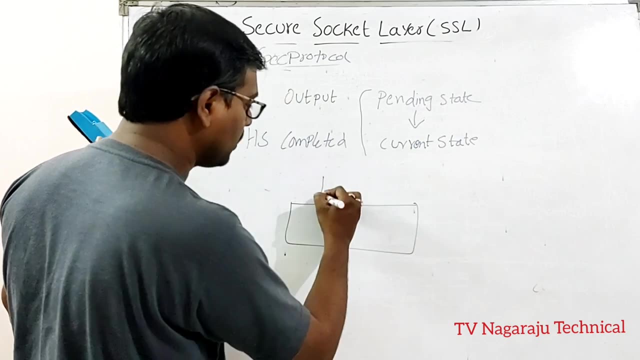 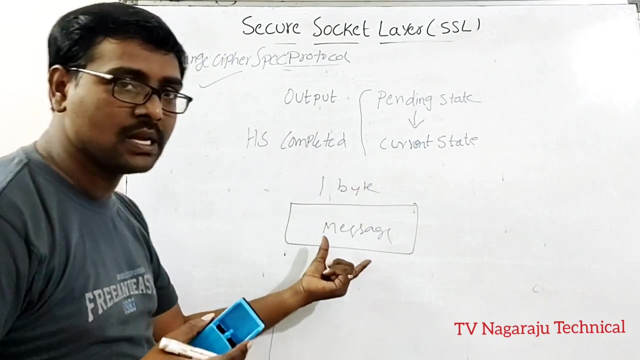 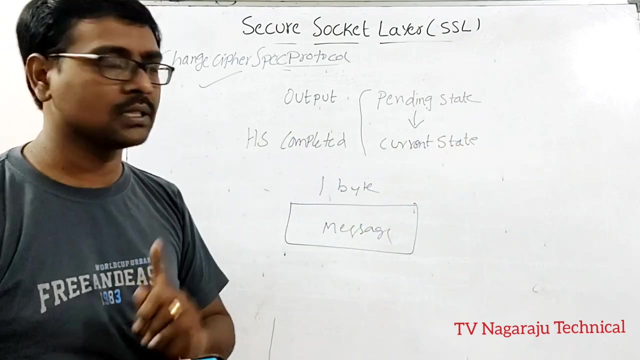 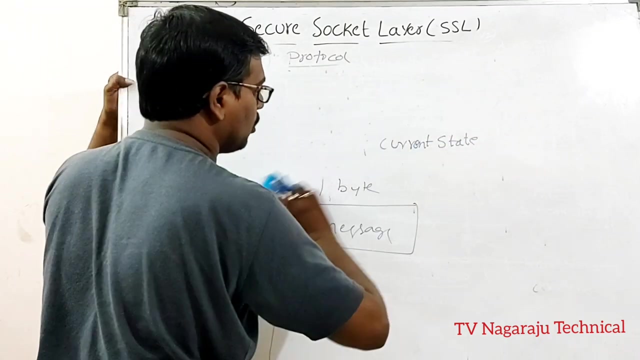 change cipher spec protocol. now, protocol converts the pending into current state, so this consists of one byte message. the chain decipher speed protocol consists of a message of one byte long. by using this one, it converts the pending into current. only one task. the purpose of this one is only this task. okay, now move to the last. 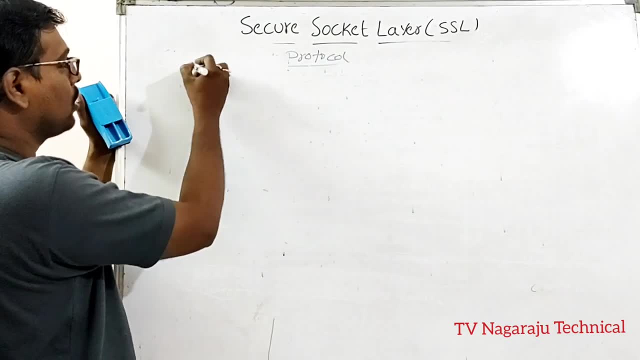 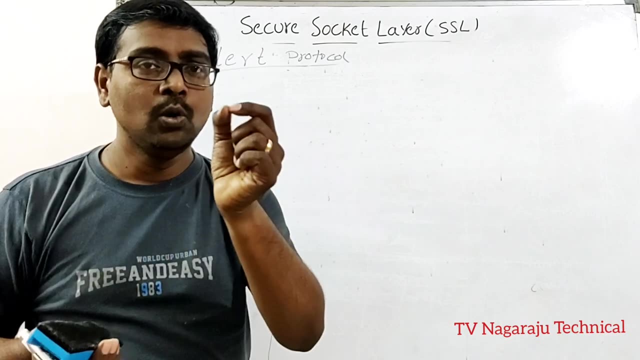 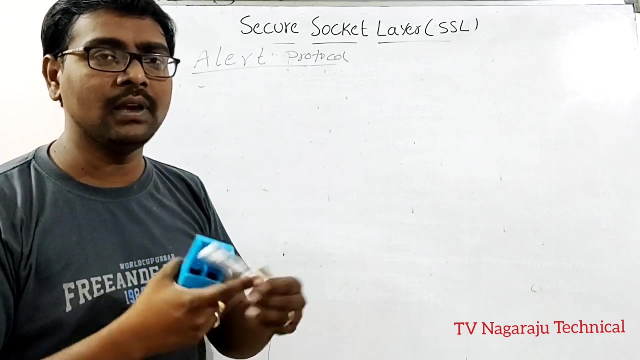 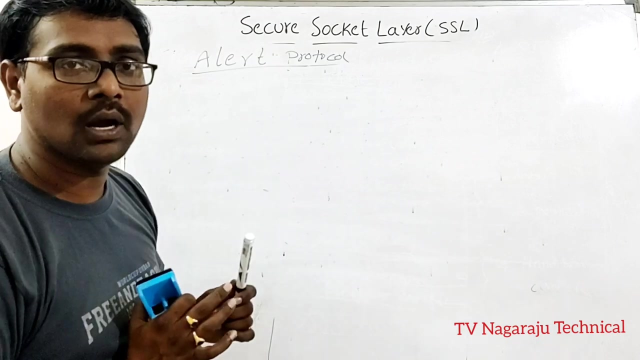 protocol. that is alert to protocol. you know the meaning alert. alert to protocol simply to convey some messages between the client and server or, simple example, to convey the messages between sender and receiver, sender and receiver: the alert to protocol is used. now the alert to protocol is divided into: 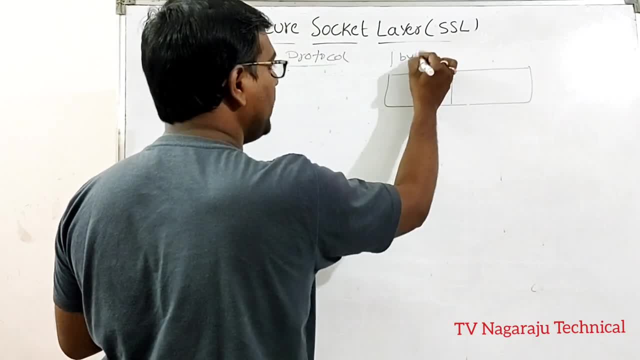 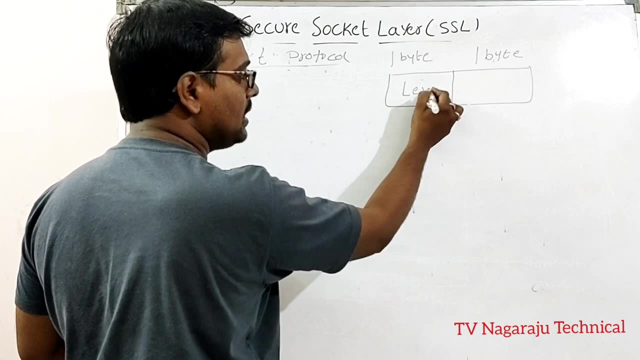 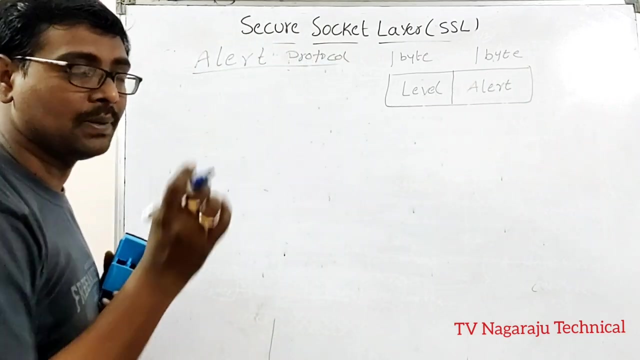 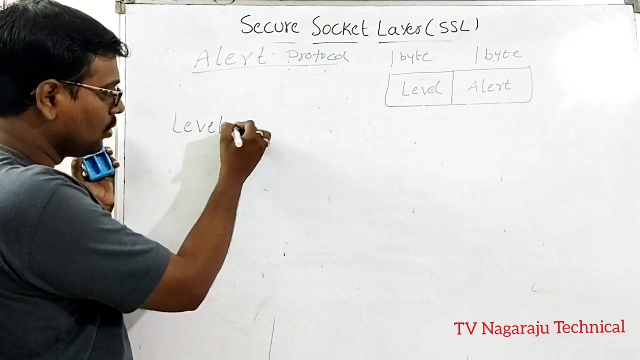 two fields. each field of size one byte. each field of size one byte. the first two field is represented by the level. the second field is represented by the alert message. two fields: level and alert. we have. level is equal to one. at the same time, level is equal to two. 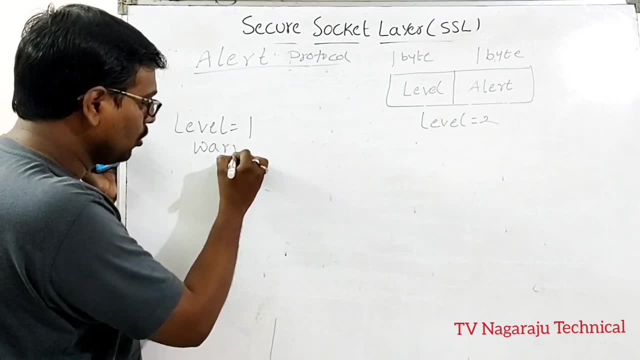 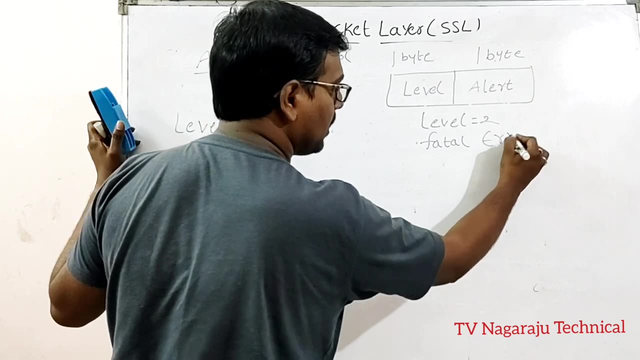 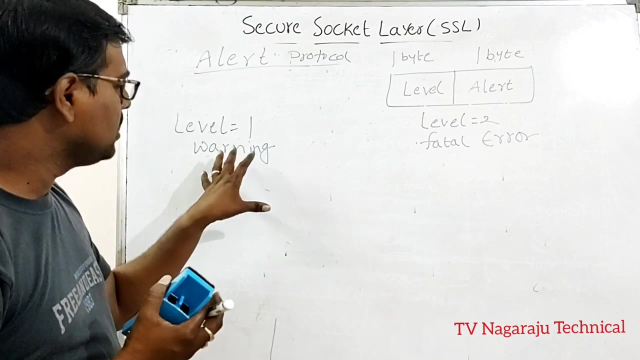 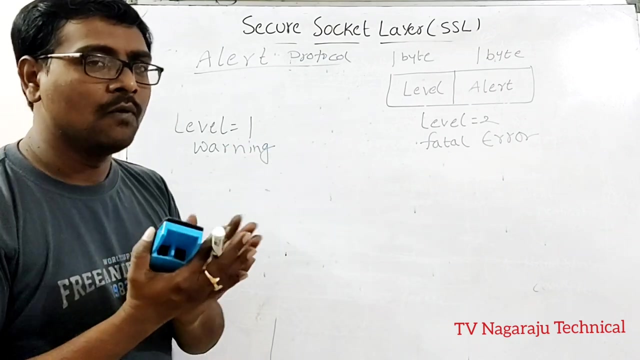 values of the level. level is equal to one means. that is called warning. level is equal to two means- that is called fatal error. what is the difference? warning, if you have warning, means there is no impact on the connection between the sender and receiver. you know the warning messages for warning: there is no impact. 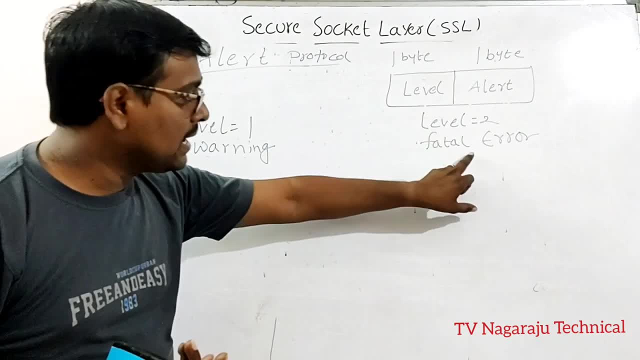 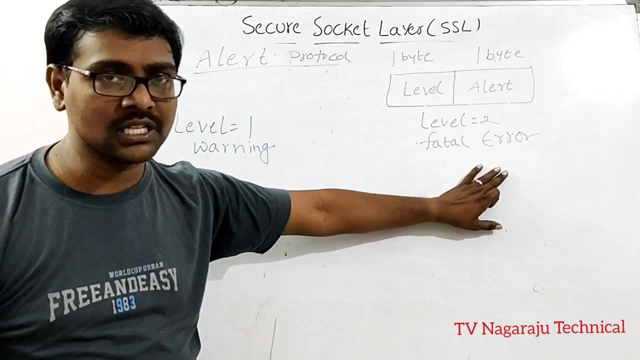 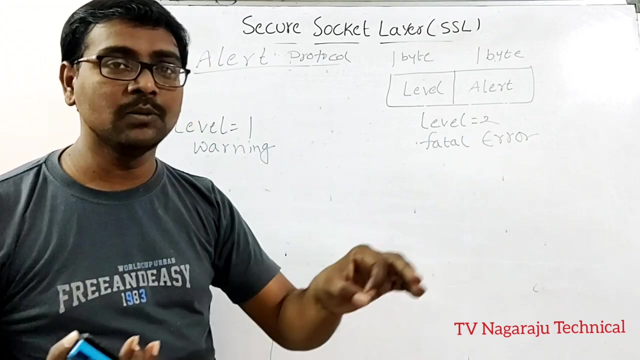 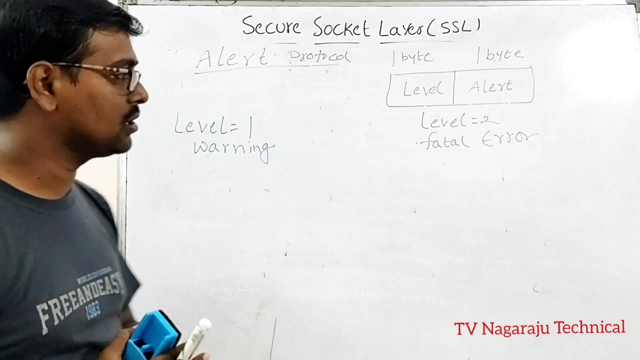 between the sender and receiver. fatal error means simply, it breaks the connection between the sender and their receiver. it breaks the connection between the sender and receiver. it is not possible to resume. if you want, you can restart the connection freshly. you want, you can restart the connection. so, based on this one, what are the different alert? 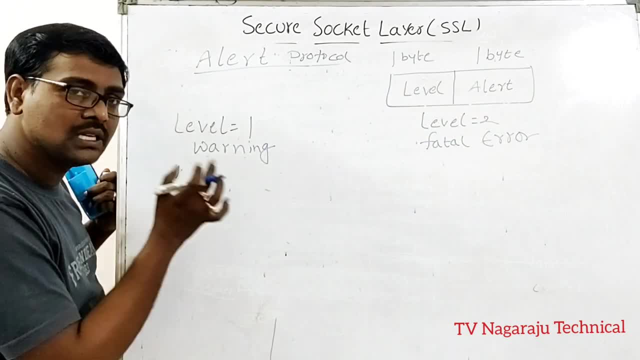 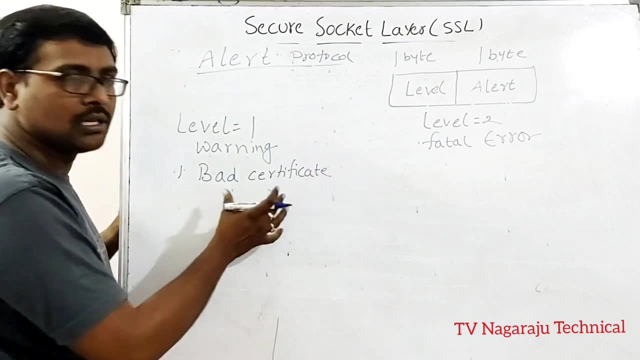 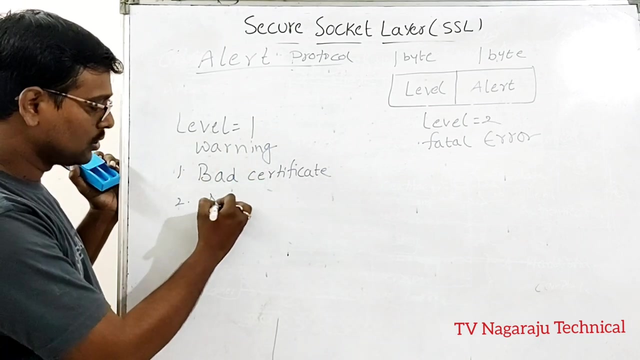 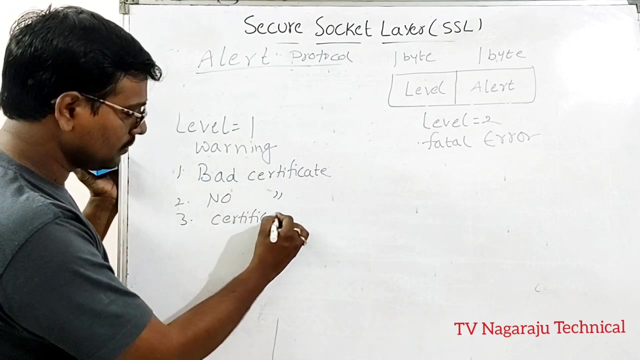 messages they provided here. every alert message related to certificates. suppose the first one is bad certificate. suppose if you have received some certificate. suppose the received certificate is corrupted or it is wrong. no certificate. suppose I am not receiving any certificate. suppose certificate expired. 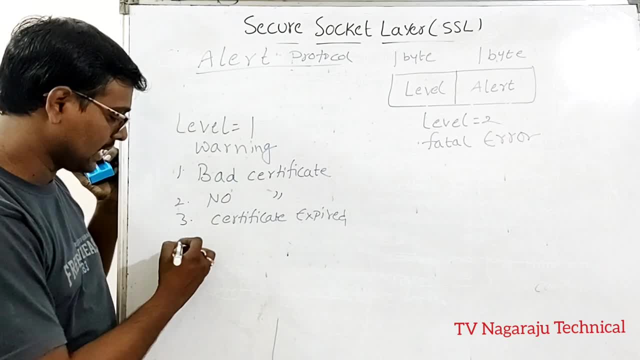 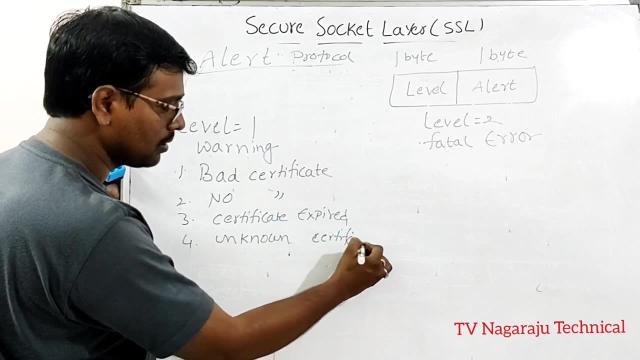 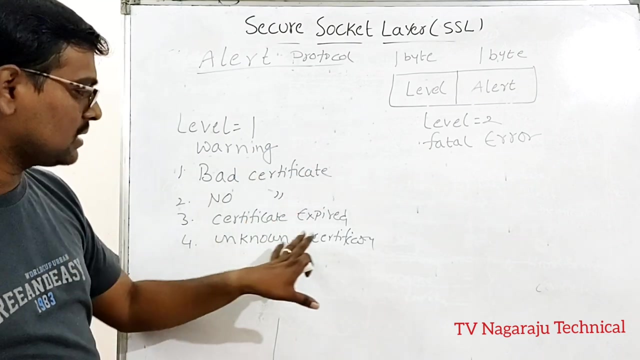 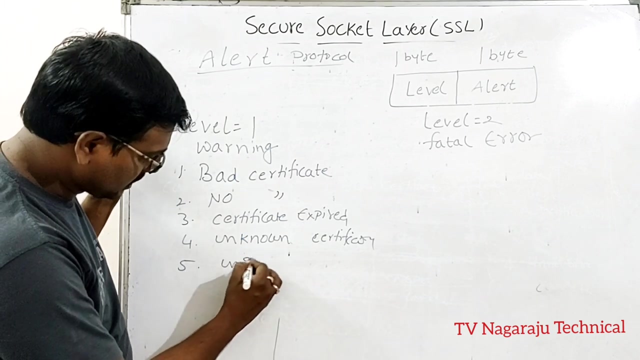 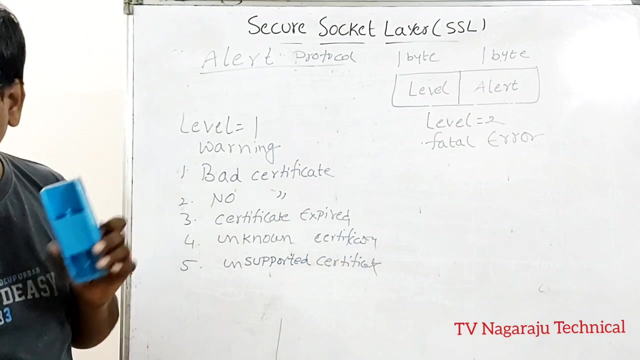 whatever the certificate I received, assume the certificate is expired. unknown certificate, unknown certificate: that is during the processing of certificate it leads to any problems, that is, the certificate is not related. now, unknown certificate, for example, unsupported certificate, so the type of the certificate is not supported. the type of the certificate is. 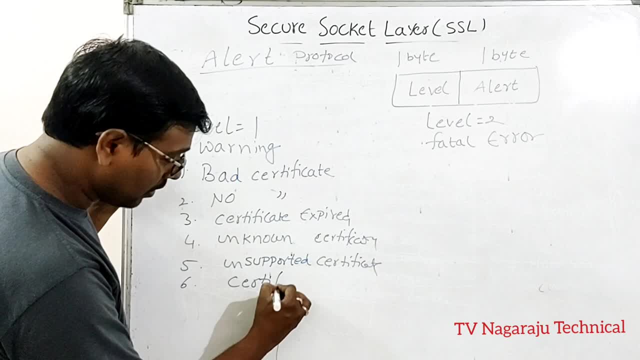 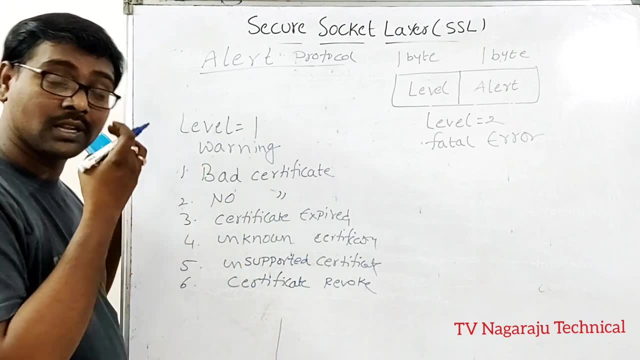 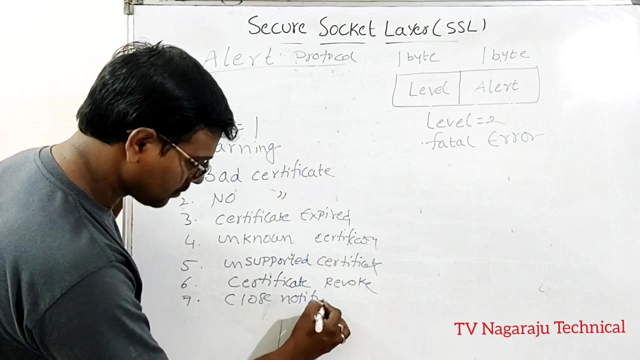 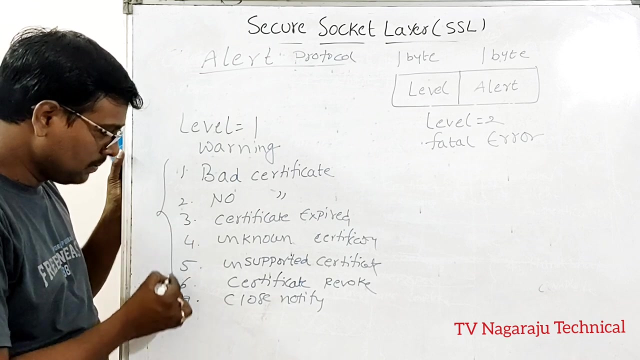 not supported. now: unknown certificate, certificate revoked. so whatever the certificate I received, that is under revocation list, that is under revocation. that is under revocation list. the next one is close notify. so close notify means the server does not want to send any messages. observe these are some warning. 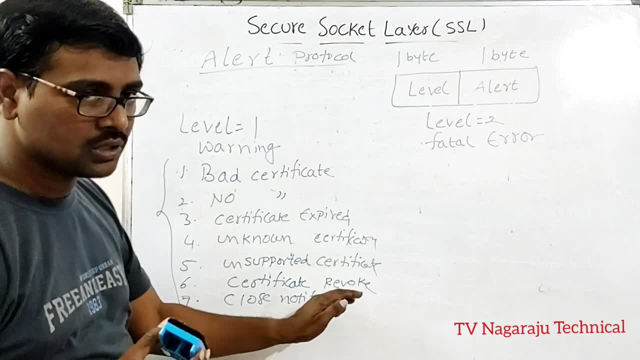 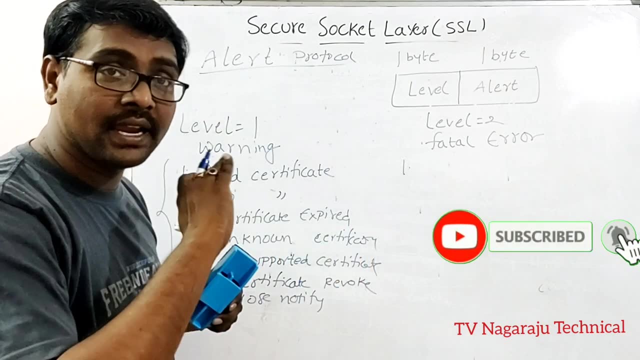 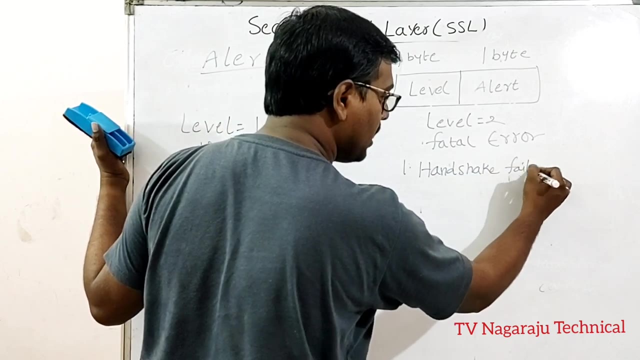 messages, even though you are getting anything related to certificate. it just leads to warning messages. but what is the fatal error? it breaks the entire connection. mean failure of handshake. handshake failure. what is mean by this one? for example, if the sender receives some illegal 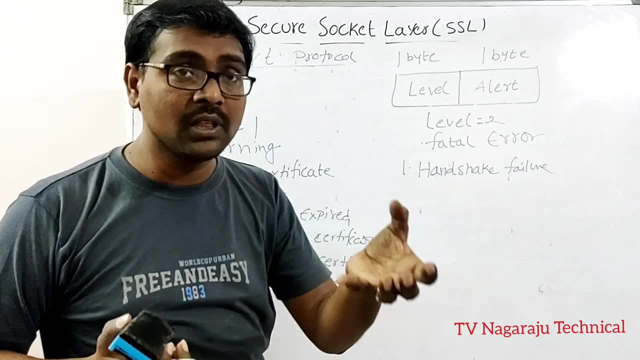 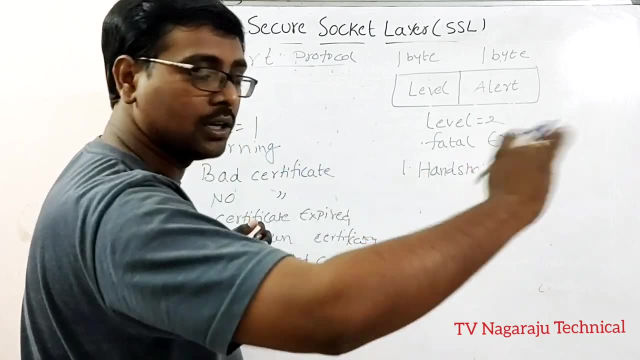 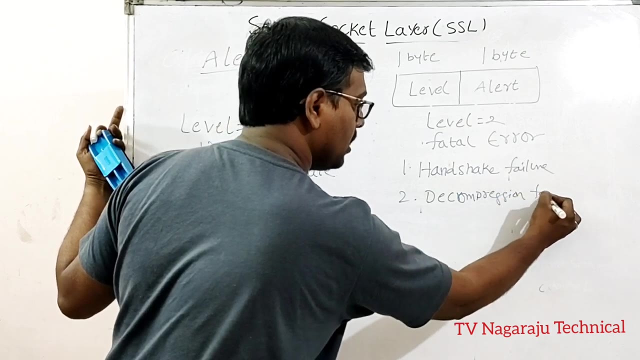 parameters. suppose the parameters that are not within the range. simply they close the handshake. they close the handshake. that is handshake failure. the connection is closed now. decompression failure. decompression failure: suppose the decompression algorithm receives the wrong. 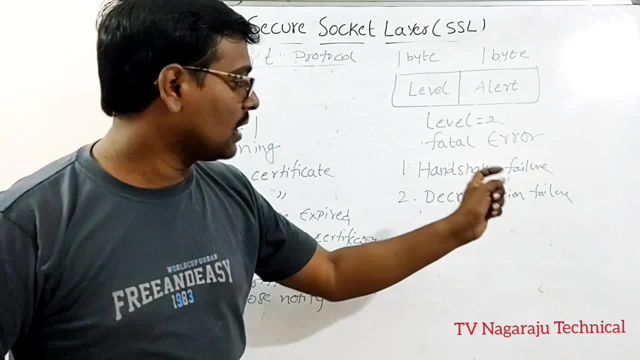 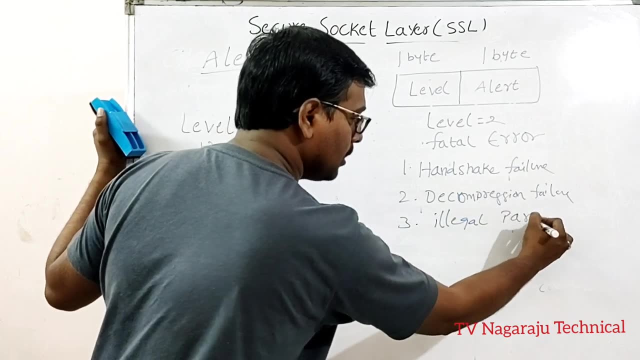 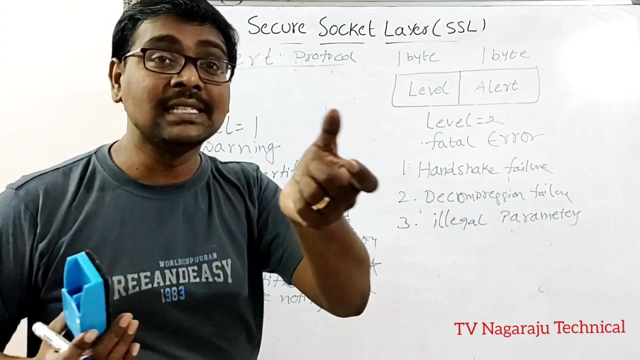 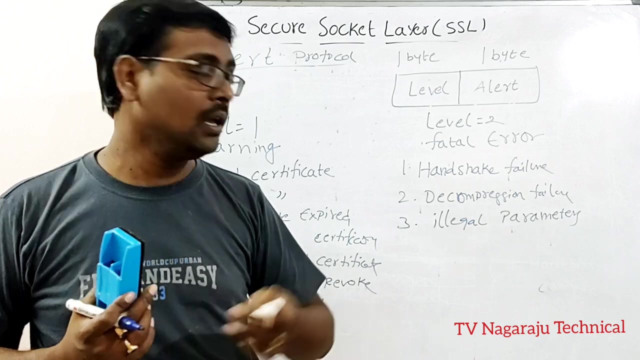 input. the decompression algorithm receives the wrong input. the connection is failed. now illegal parameters. illegal parameters: suppose the parameters what we are received, those are inconsistent, the parameters are inconsistent and can be negligible to any insecurity. though, simply the handshake, simply the connection. 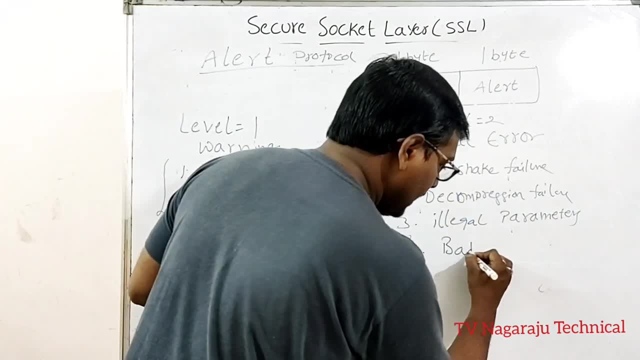 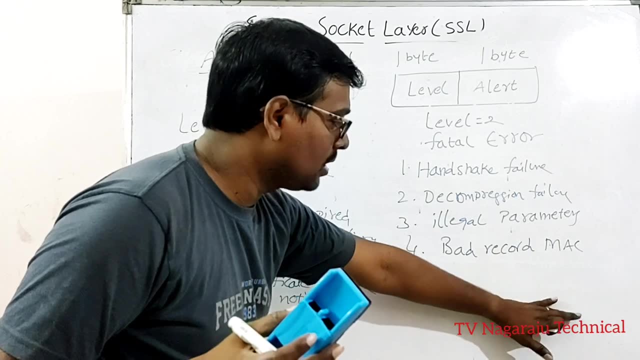 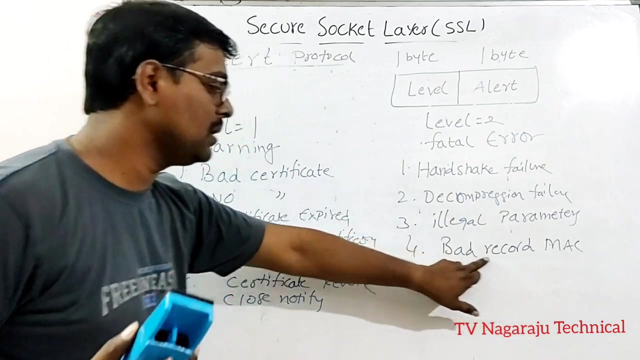 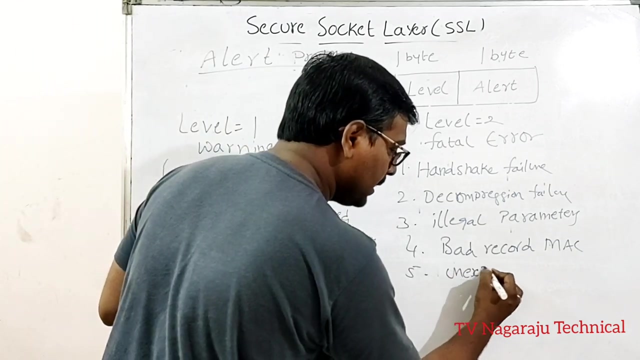 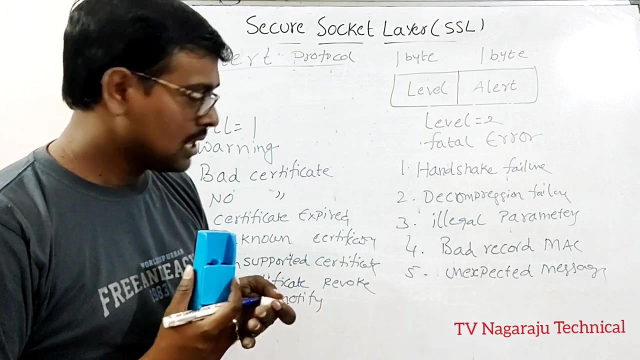 is closed. next one is bad record: MAC. so receiver or sender receives the message authentication code. suppose if the received message authentication code and the original one both are different, that means whatever the record we are received, that is the bad record. Finally, unexpected message: suppose we are receiving a message not related to this connection. 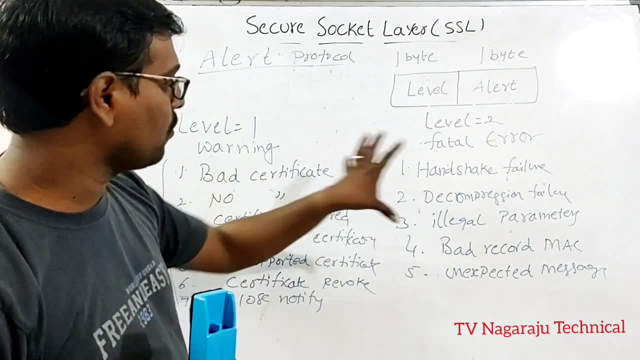 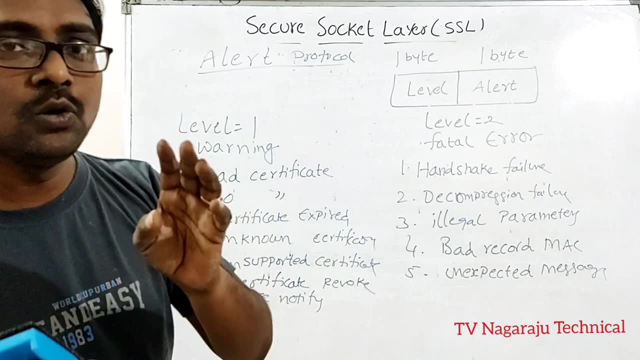 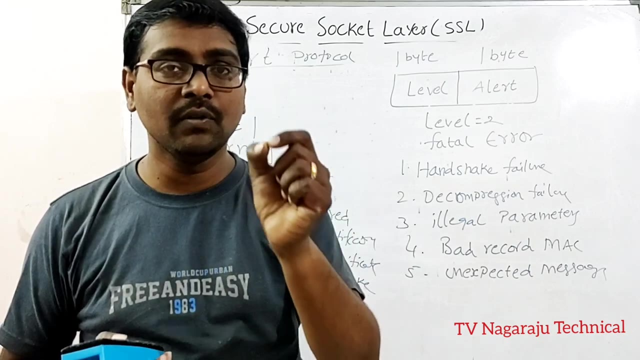 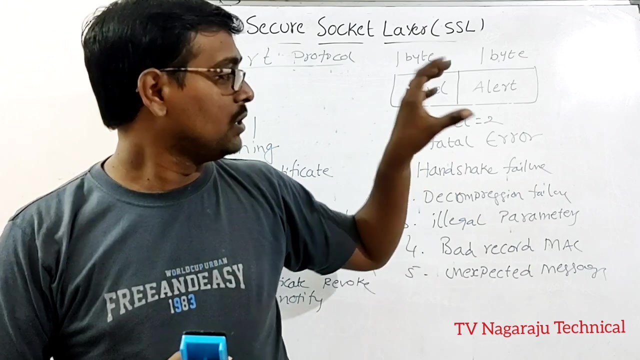 simply close this one. these are different types of warning messages and fatal errors. finally, this is called secure socket layer. so secure socket layer is simply used to provide security to the data that is transferred between the client and server. it consists of four protocols: SSL record protocol, which is used to generate some output based on that one. 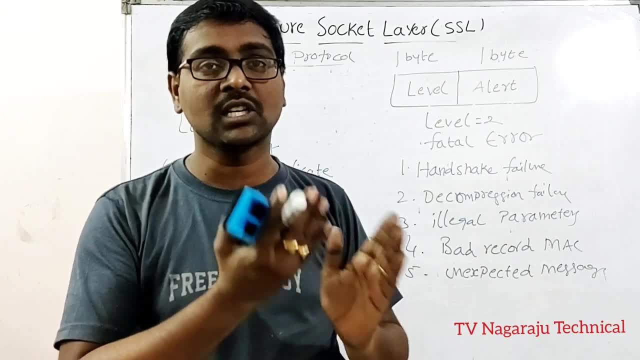 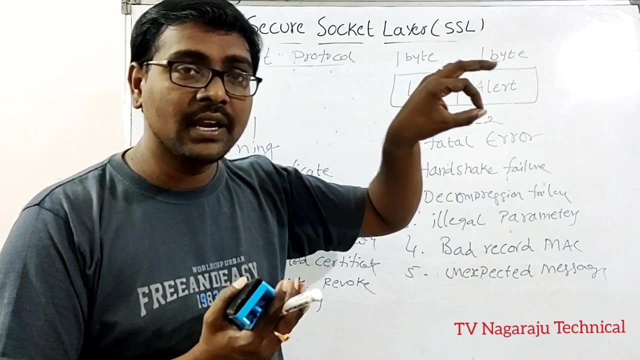 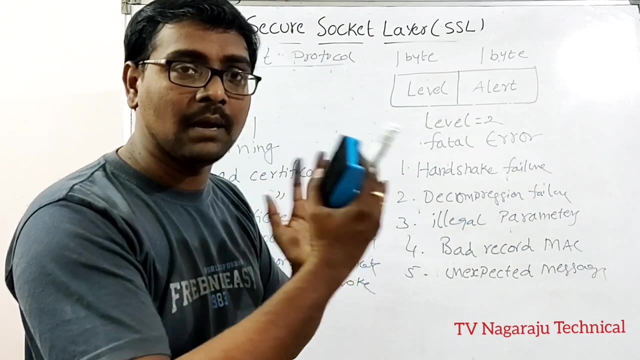 handshake protocol, which is used to establish session among the client and server. change ciphers way protocol to convert the output generated in the SSL from the pending state into current state alert protocol: simply convey the messages, that is, alert messages, between the sender and receiver. 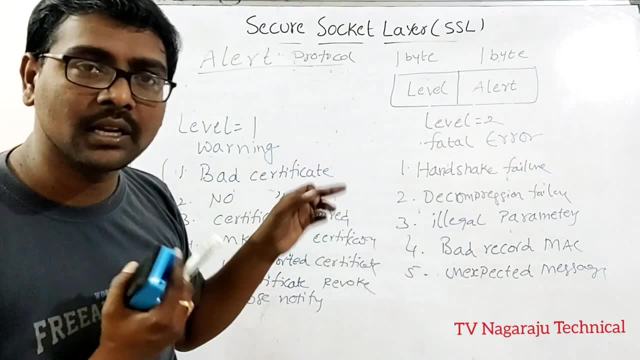 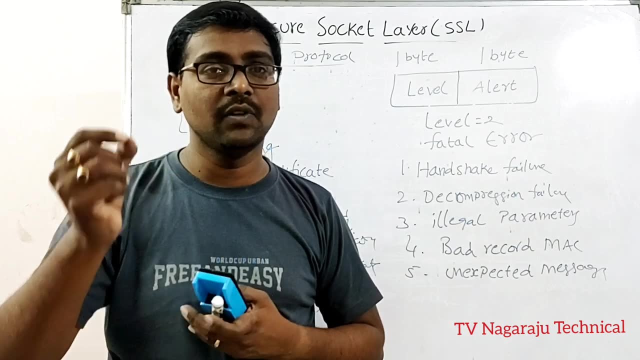 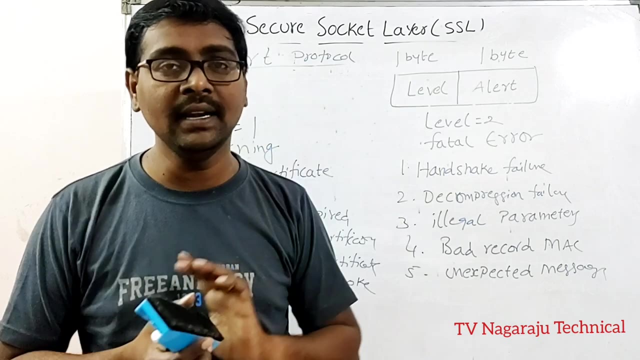 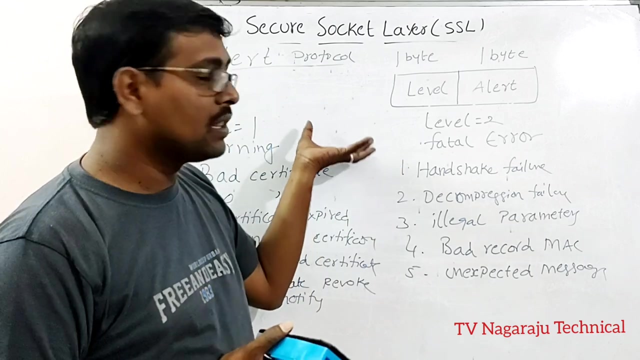 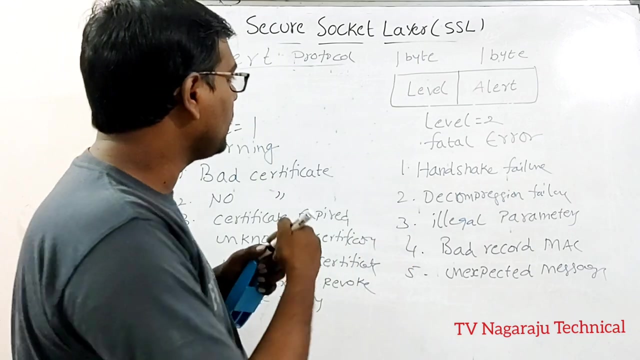 So when we enter this, we are regularly using the term certificate. What is mean by SSL certificate? Simple for your understanding: SSL certificate is a digital certificate used to secure and verify the online transactions. Secure and verify the website. Secure and verify the data that is transferred to the online transaction. Each and every certificate is issued by the certificate authority. 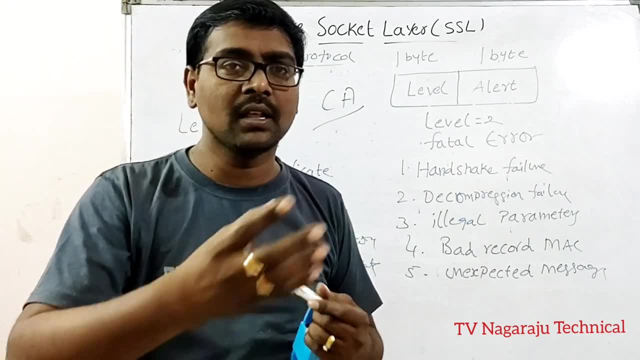 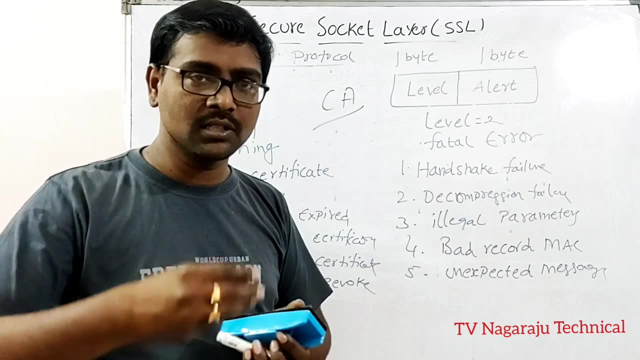 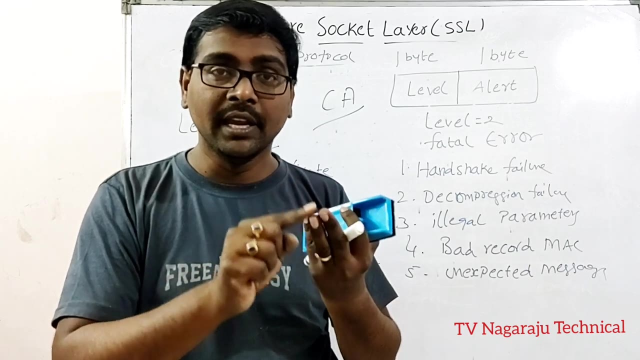 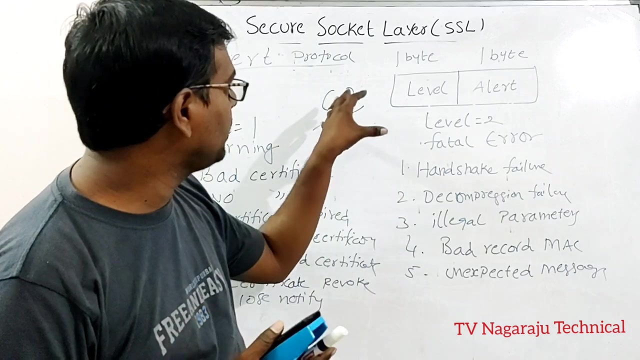 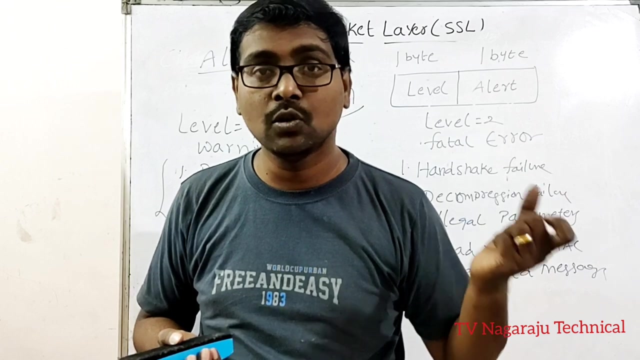 Before issuing the certificate by the certificate authority, it verifies the website. If everything is okay, then the certificate is issued. What are the characteristics? Because of that certificate, it provides the encryption. The certificate consists of encryption, integrity, authentication, non-reputation, public key exchange. Everything is maintained during certificate. So you already know the concept: How to create a certificate. Example: X.509 certificate Like this. only This is secure socket layer. Thank you very much.